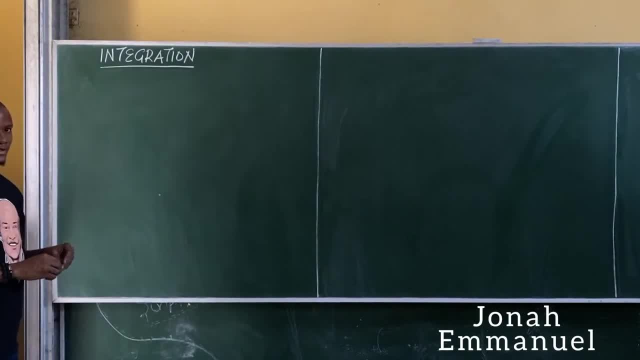 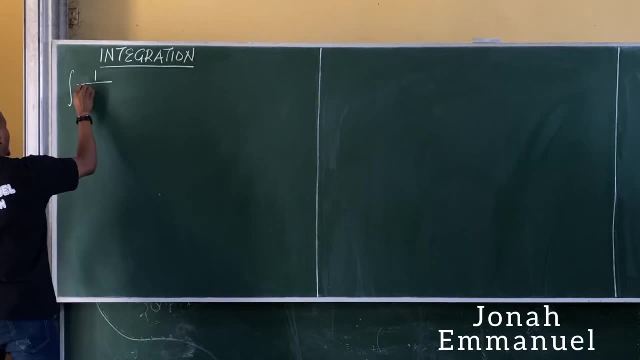 to do this. So for this case, note this. Let's say, if I'm given to evaluate an integral of the form, integral of 1 over a squared plus x squared For an integral of the form a squared plus x squared to x, the solution to this would be to substitute the value of 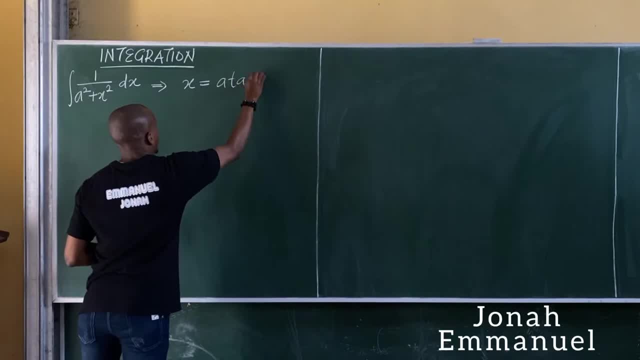 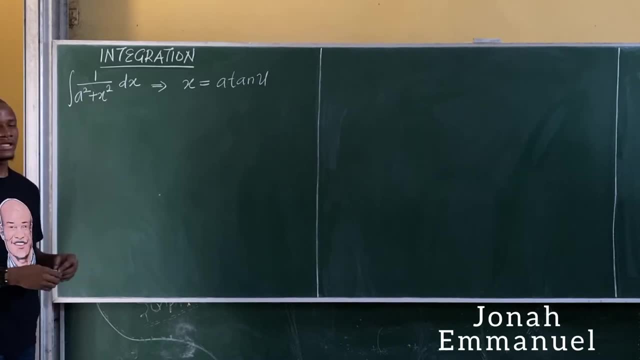 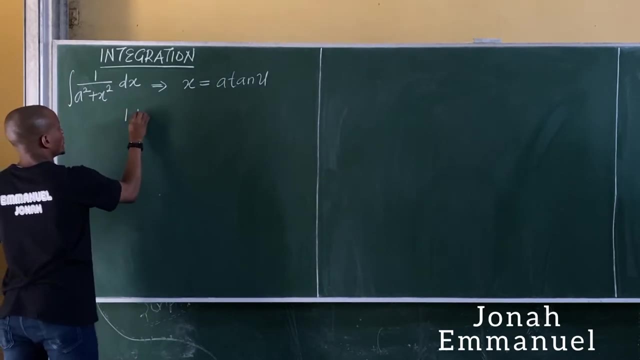 x as being equal to a times u. This becomes the idea towards solving equations of this form. Let's say it's equal to a times u, And also remember the trig ratio or the trig identity that says that 1 plus tan squared x is equal to sin squared x. So these are: 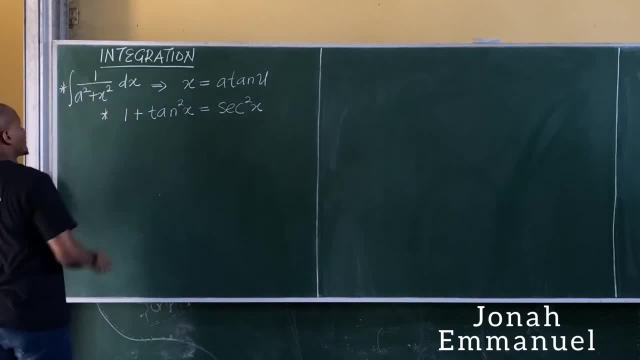 like the key points of integrating or of evaluating integral of this form. We'll take an example and see how we work on this Example. Let's say I'm asked to integrate 1 over 9 plus x, squared Of course yes, Evaluate this. Alright, for this now looking. 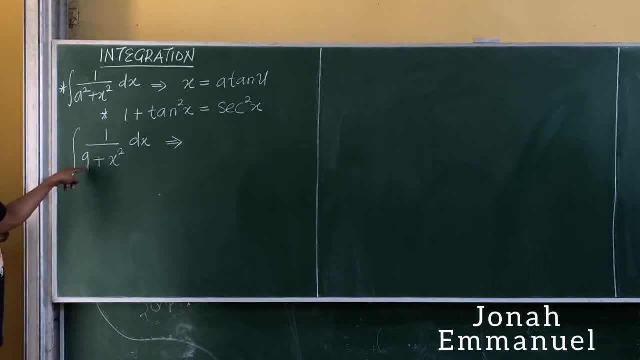 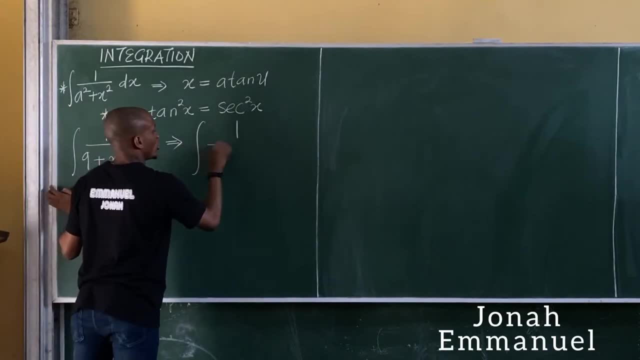 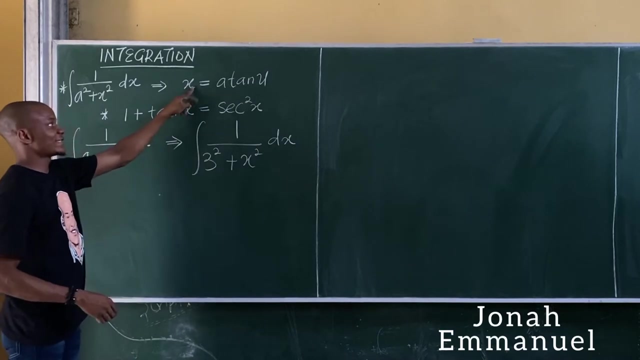 at this equation I know that I can express 9 in terms of 3, because 9 becomes 3 squared. So this now becomes the integral of 1 over 9 is 3 squared plus x squared and there the x. So in an integral of this form we said: put x as a times u where a is the term that's. 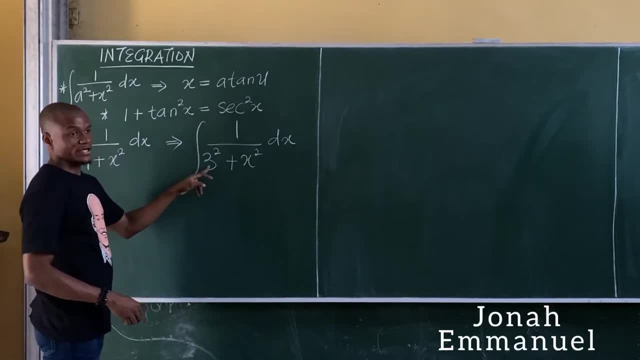 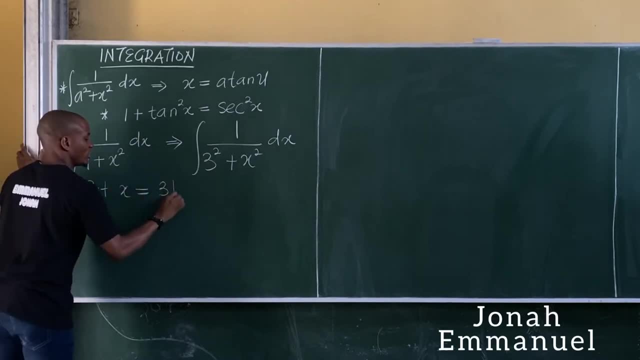 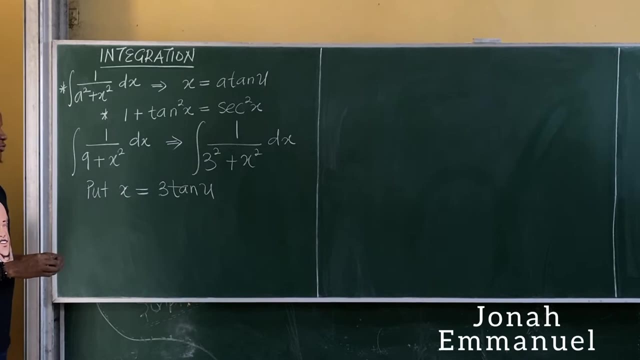 being squared. In this case, now, the term being squared is 3.. So I'll now say: put x as being equal to 3 times u. The first case now would be to find the value of u alright, or make u subject of the formula. If I'm to make u here as the subject of the formula, 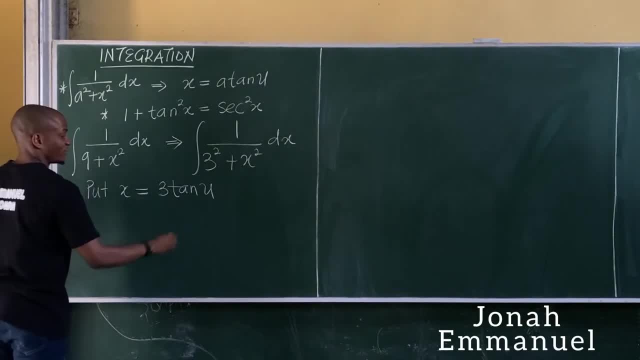 case 1 would be to divide both sides by 3.. If I divide both sides by 3, x- all over 3 would be. here would now be equal to if I divide here by 3,. 3 cancels 3, I'm left with tan. 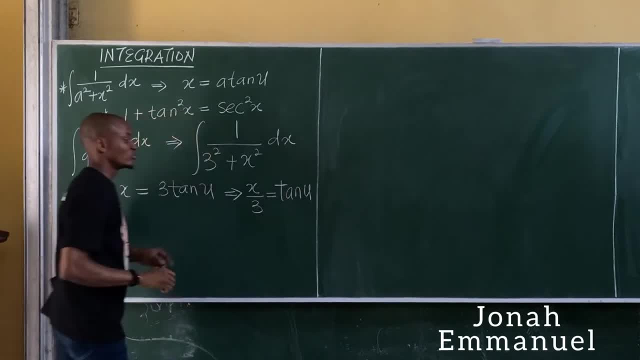 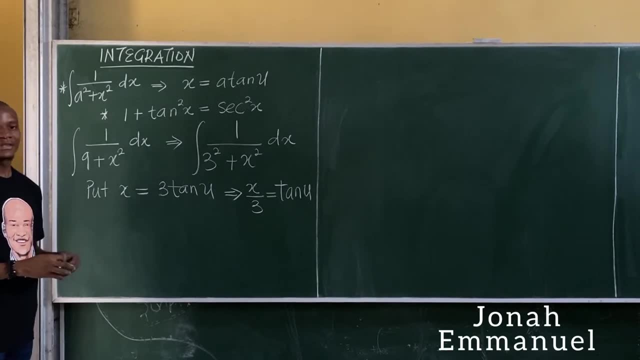 u. This becomes tan u, So x over 3 equal to tan u. Let's get u. How do we get u now? Divide both sides by or take the tan inverse of both sides. If I take tan inverse of tan u, 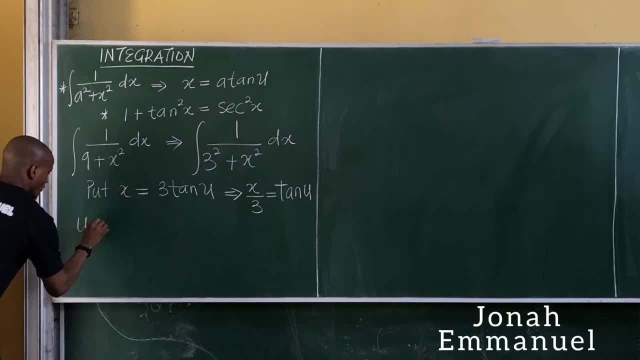 I'm left with u, So hence u is now equal to. if I take tan inverse of this, it becomes tan inverse of x all over 3.. So I have this. So I have u as being equal to the tan inverse of x all over 3.. My next step would be this: If I have, you could have said I had that. 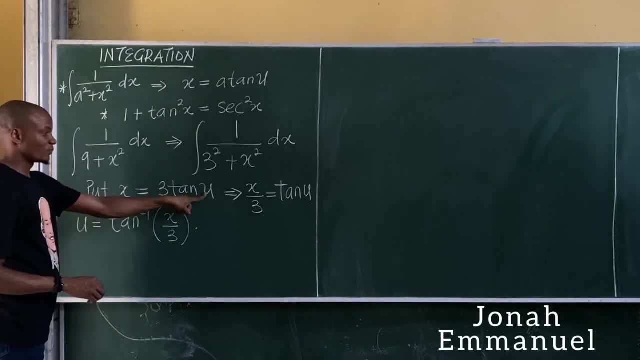 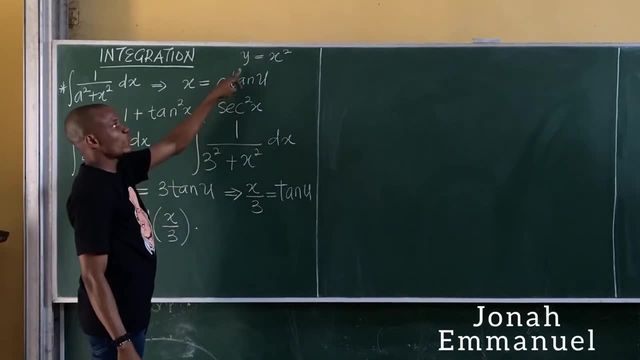 x is equal to 3 tan u. If I, if I have y per c being equal to 3 tan u, then I would have x being equal to x squared. If I differentiate y with respect to x, I would get the y over. 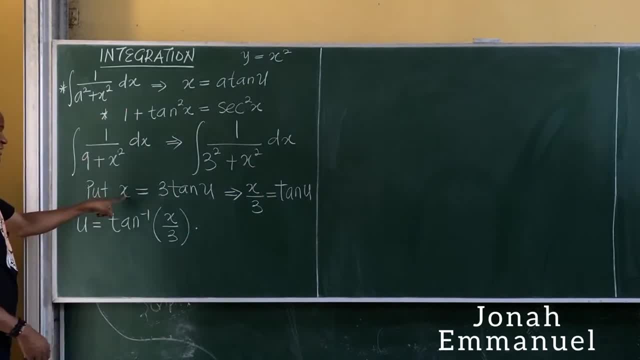 the x In the same case. if I differentiate, in this case now I'm having x being equal to 3 tan u. If I differentiate x with respect to u, I would now get the x over the u, Just like when you had the y over the x. in this case, it becomes the x over the u To differentiate. 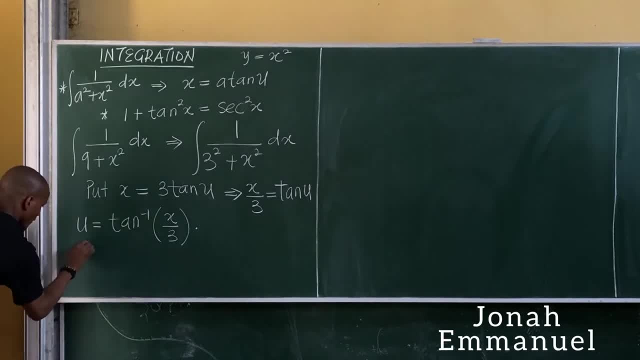 x with respect to u, I would get the x all over. The u is equal to. if I differentiate 3 tan u, I would get 3.. Differentiate tan: you get x squared And of course you have u. So this now is from this: Differentiate x. 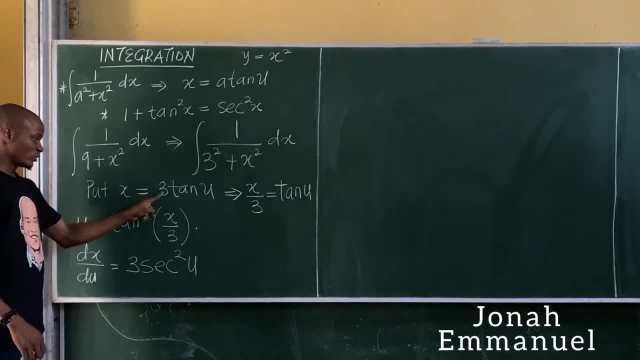 you get 1,. the x by the u is equal to your constant 3.. Differentiate, tan u. you get x squared u from differentiation. Alright, from here. now what's the x From the y? now I can see that the u goes this way. now I'll have that be x. So the x is now. 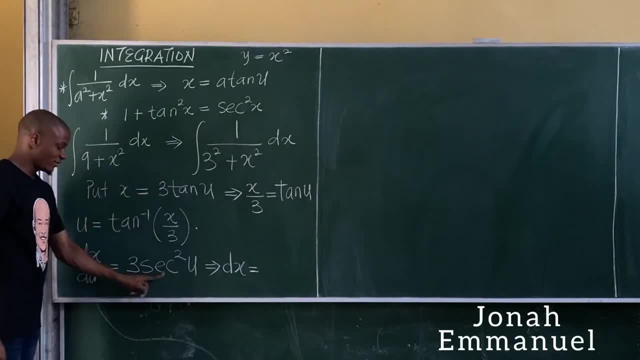 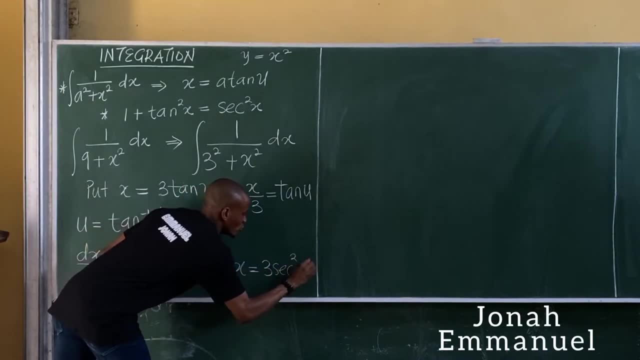 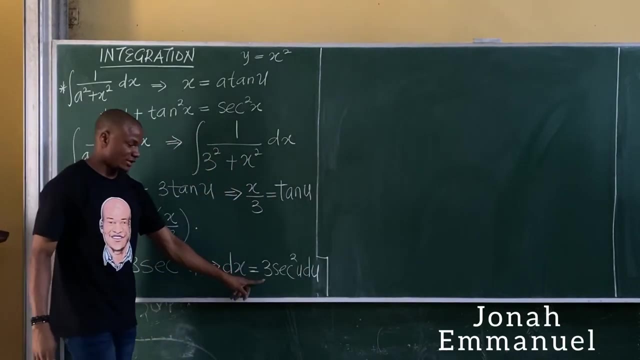 equal to the u goes this way: I'm having 3 tan u, then the u, So 3 tan u and then the u. So this is the value of the x. The x is 3 tan u, the u. Alright, at this point. 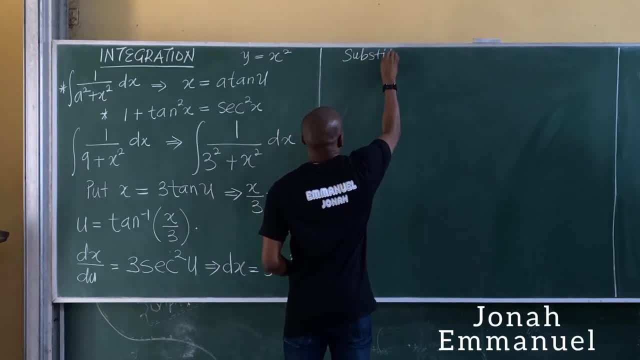 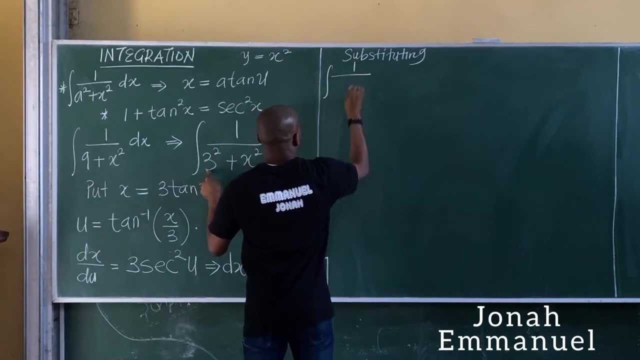 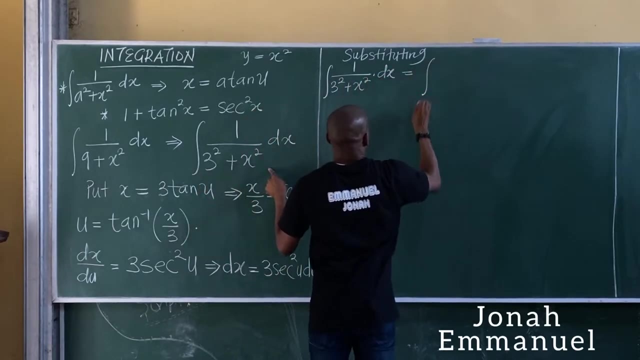 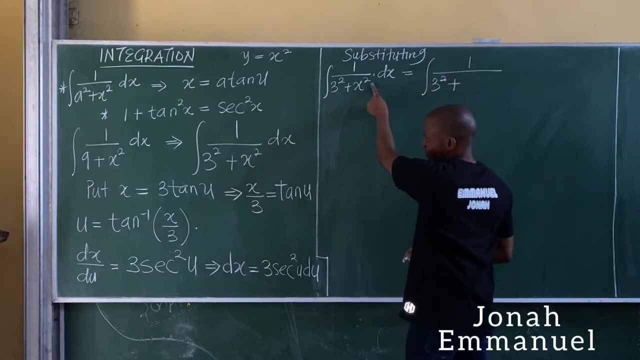 now substitute u. I have that the integral of 1 all over 3 squared plus x squared dot gx will now be equal to integral of 1 all over. this gives me 3 squared plus. I'm having x squared. What's x? x here, we said, is 3 tan u. that's one of x here. So in place of x here I'm. 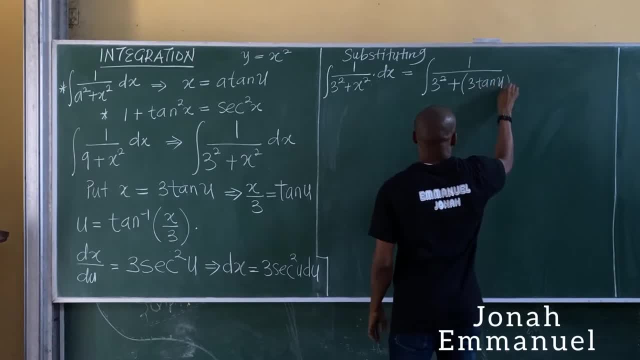 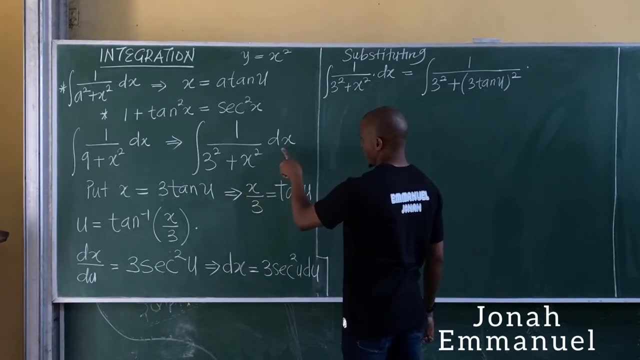 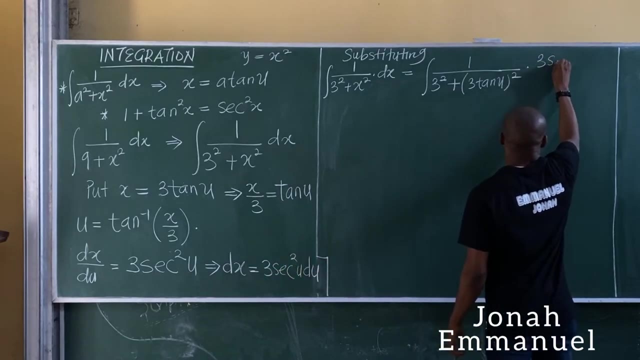 going to put 3 tan u. This is now x all squared dot. next up is the x The x, as we said here is 3 z squared u the u. We call it 3 z squared u the u. Alright, so this is now the value. 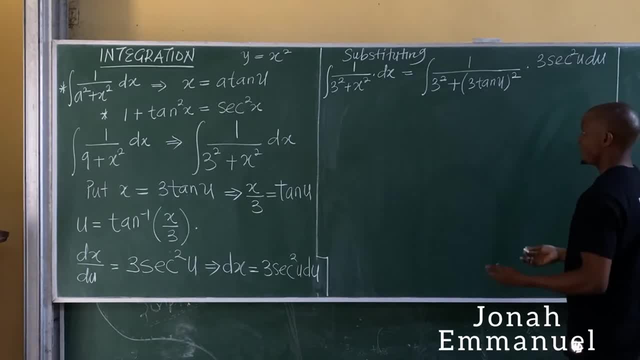 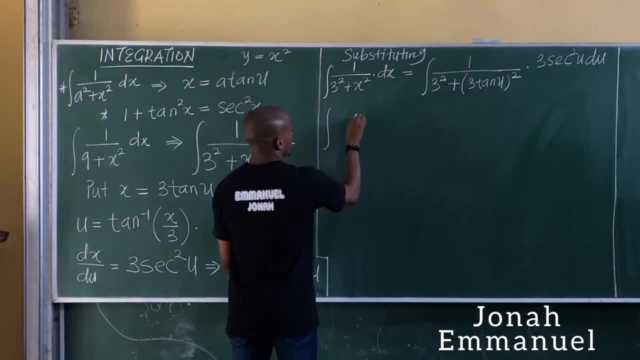 of x. How do we work on this now? My first task now will be expand this. If I expand this, I will be able to expand this. I will be able to expand this. I will be able to expand this. I will now have integral of 1 all over. this gives me 3 squared plus. this now is b squared. 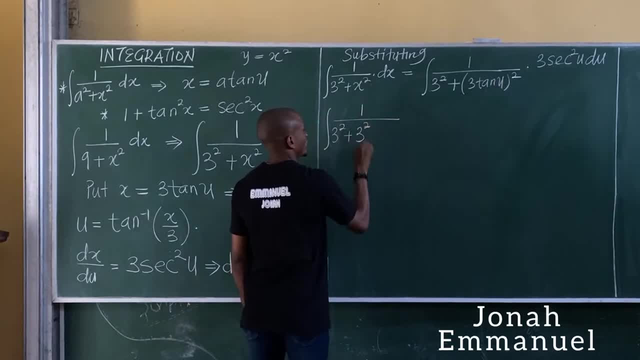 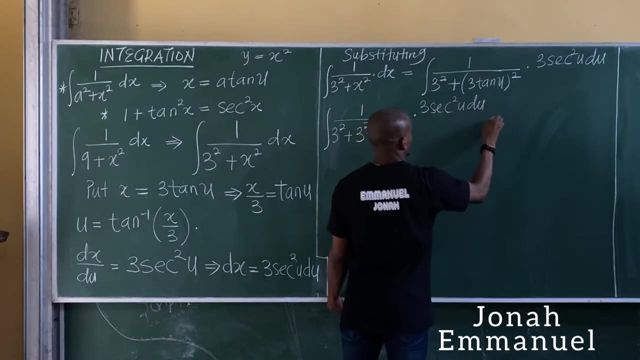 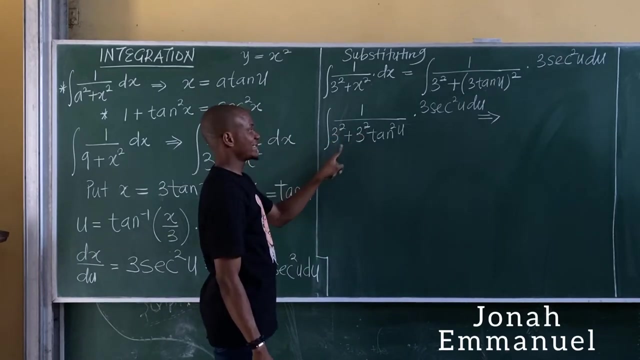 So this is 3 squared. I'm having 3 squared into tan? u. all squared is tan squared u. So tan squared u dot. this is now 3 z squared u, then the? u. I have this Next up. I can see 3 squared. I can see 3 squared, So hence I can factorize 3 squared. 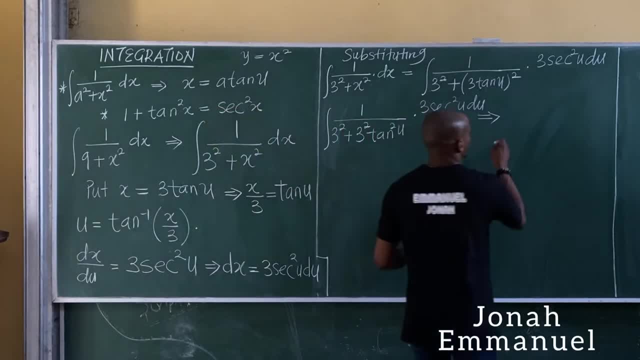 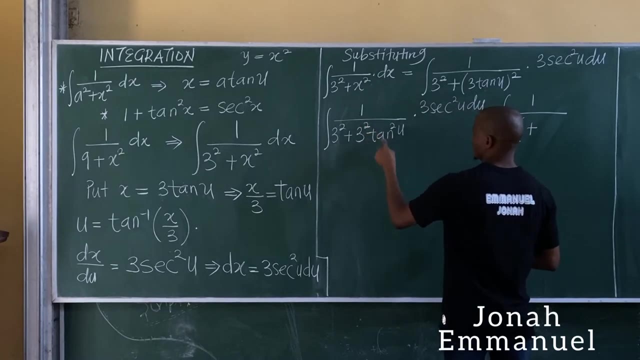 here. If I factorize 3 squared here, I'll be having the integral of 1 all over. take out 3 squared, I'm having 3 squared. Alright, 3 squared divided by 3 squared here gives you 1 plus 3 squared tan squared u divided by 3 squared. 3 squared will come to 3 squared. 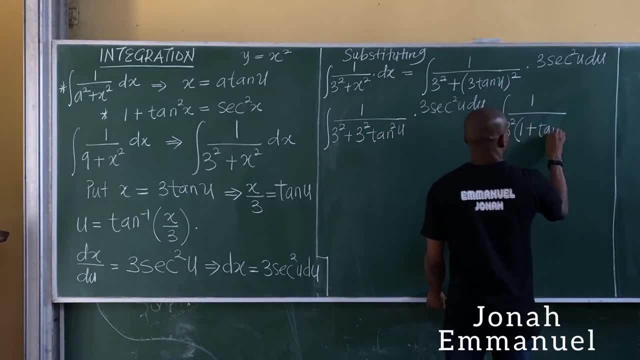 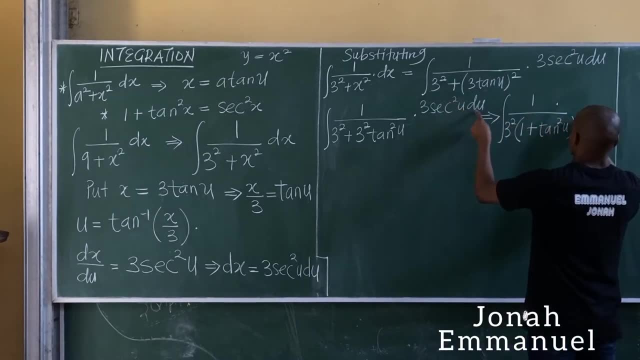 I'm left with tan squared u, So plus tan squared u, I have this Dots: I'm having 3 z squared u, du, 3 z squared u and then du Yeah, Alright, so I have this as what I have here. 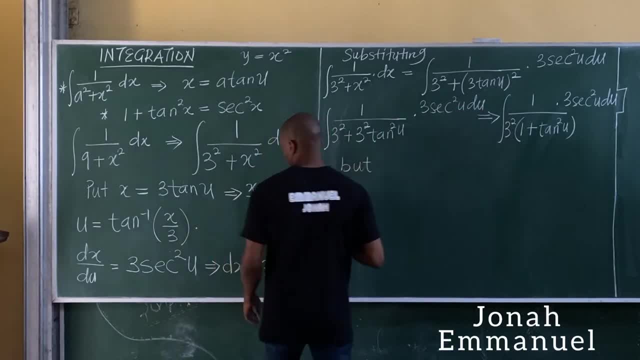 Alright, but but from these three functions we said 1 plus tan squared x is equal to z squared x. So this is u now, Hence I'll have that. in the same manner, I'll have that 1 plus tan squared u is equal to z squared u. So got, 1 plus tan squared u is equal to. 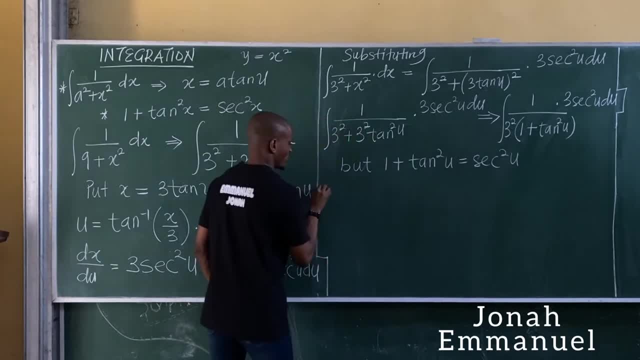 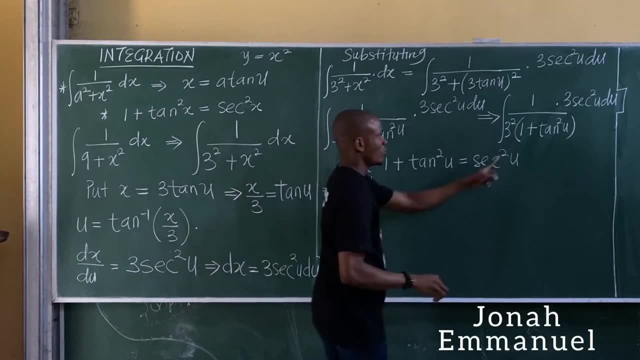 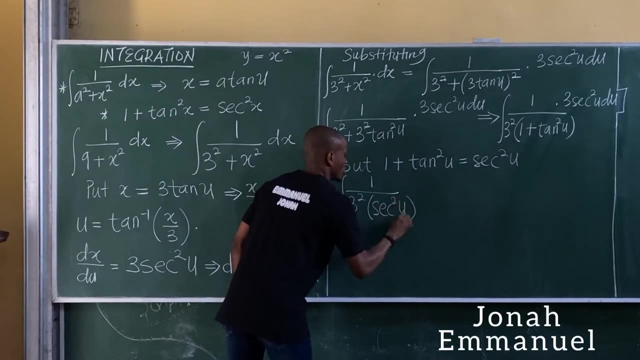 z squared u. So hence this now becomes an integral of 1, all over 3 squared. Now we're having 1 plus tan squared u. We just said 1 plus tan squared u is equal to sex squared u dot. next of this. 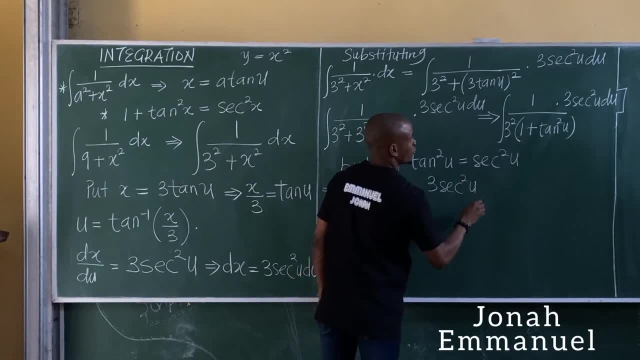 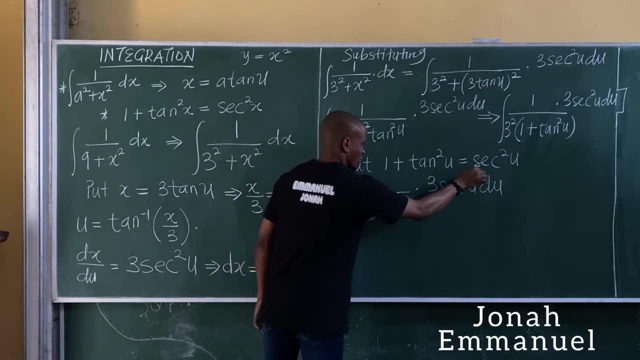 3 sex squared u. and then du, What would get is this: I can see: sex squared- cancels sex squared u. right, Sex squared u cancels sex squared u. This is 3 squared, This is 3.. So 3 here, 1.. 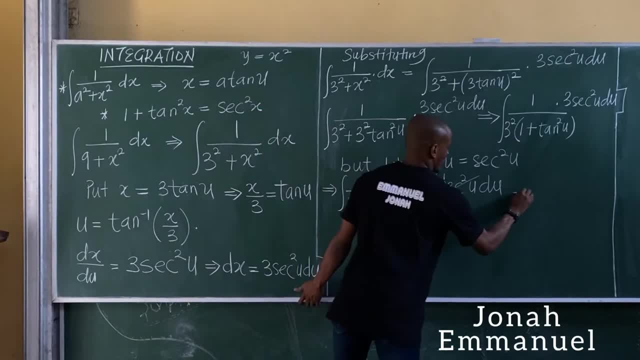 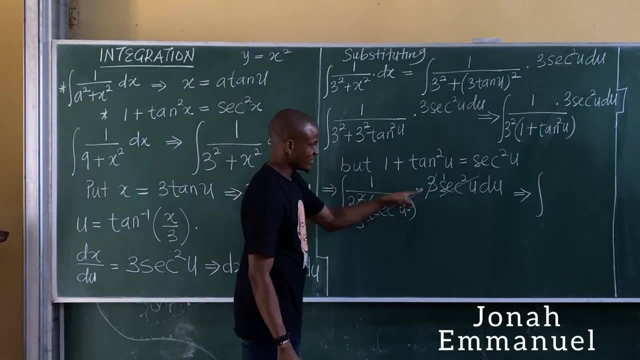 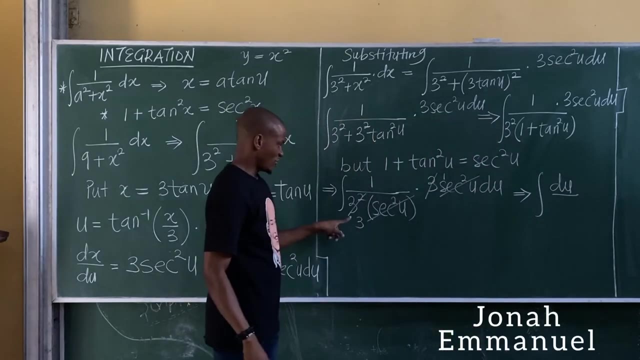 3 here I'm still having 3.. So this will now be equal to integral of 1 times everything here is gone. 1 times du gives you du 1 over. what I'm left with here is 3.. So 1 over 3.. 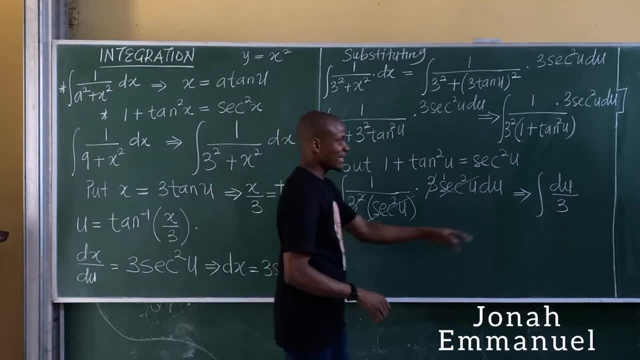 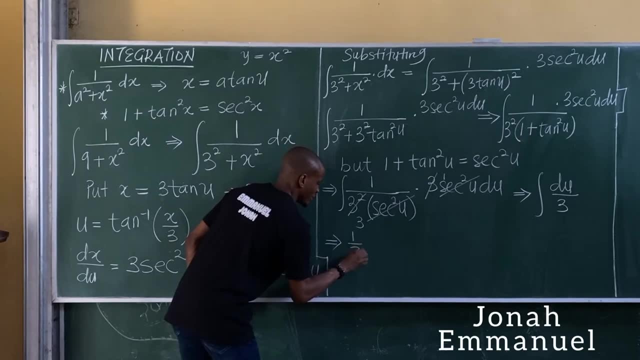 So in essence this is now equal to my constant here is now 1 over 3.. So take 1 over 3 outside the integral side becomes 1 over 3. Integral- I'm left with du. okay, Take 1 over 3 outside the integral side. 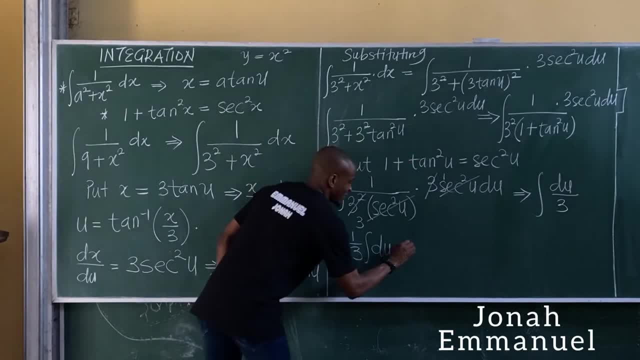 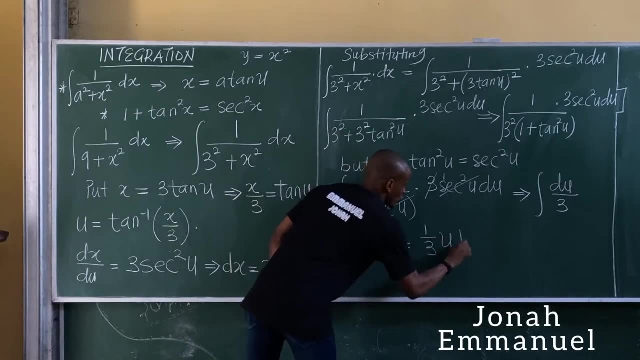 I'm left with du, So I have this. If I integrate du, I'll get u. So this gives you 1 over 3. integral of du gives you u plus c. Alright, but we have a value for u. We said u. 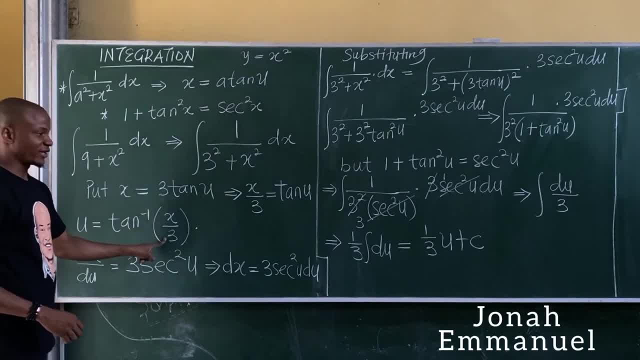 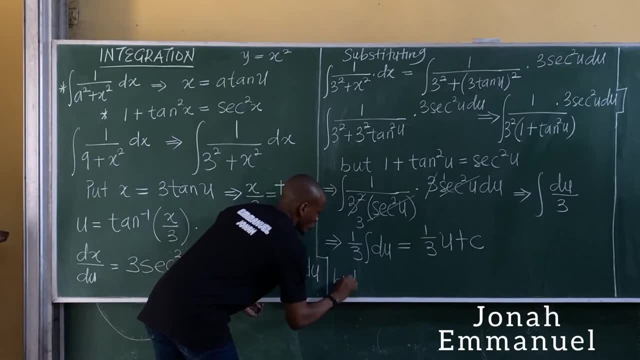 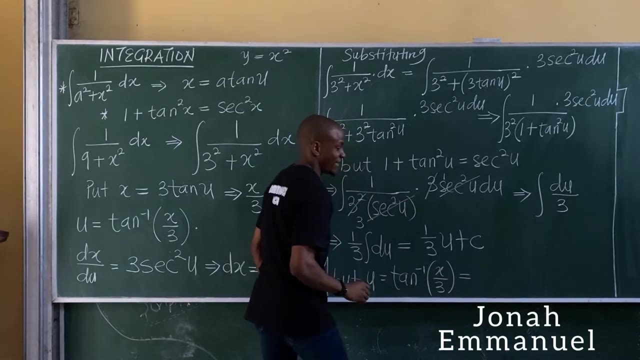 is equal to what there Tan inverse of x over 3.. Alright, so put the value of u here. So therefore, we said u, but u is equal to tan inverse of x over 3.. So therefore, my final answer is 1 over 3. 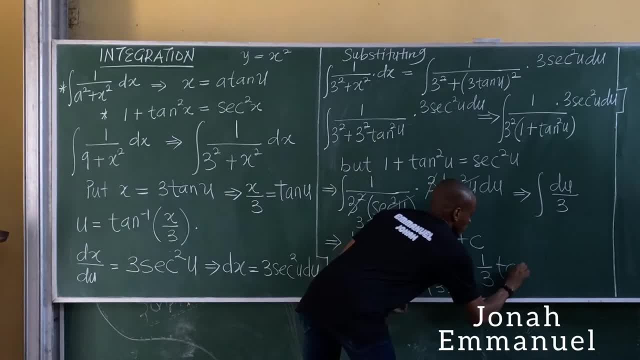 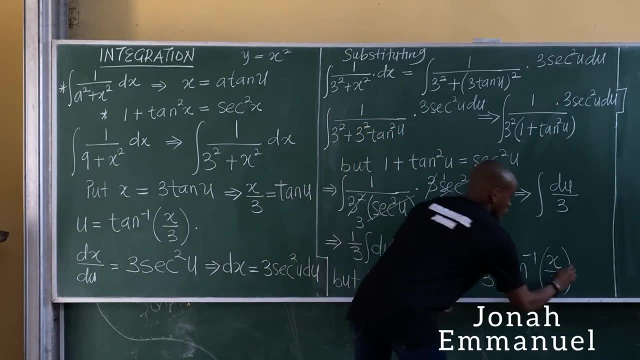 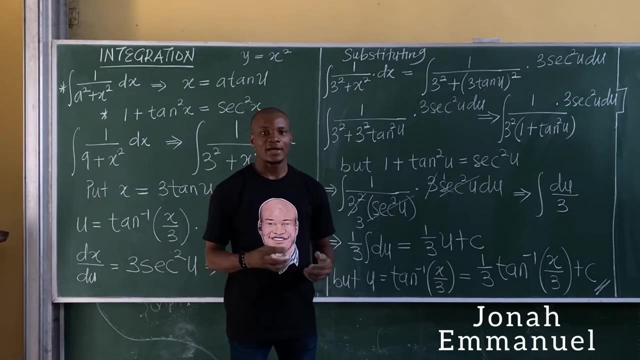 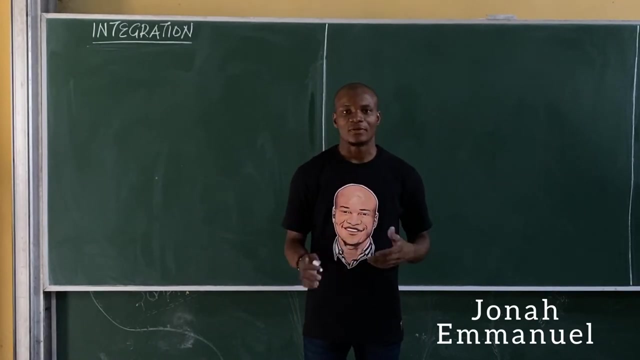 into u. u is tan inverse of x, all over 3.. This, that's u plus c. So plus c, which is the constant of expression. So this becomes my answer, after integrating. So let's go back. The second case of method of substitution. 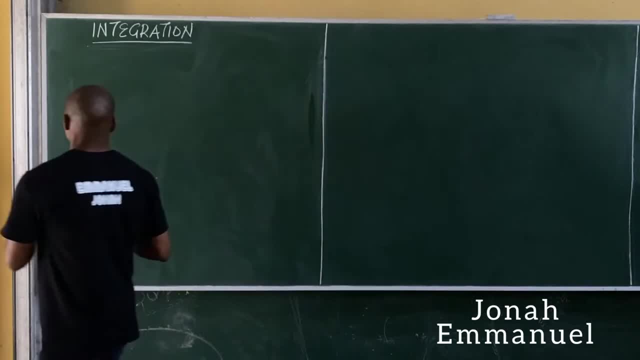 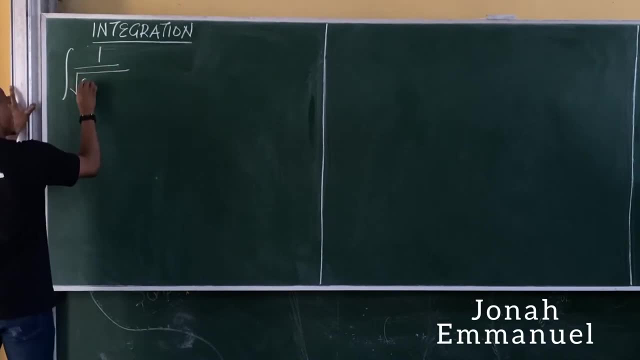 involving three functions. The case 2 is this: If I'm giving the value of an integral in the form 1 all over root, a squared minus x squared, In this case, of course, let's say it's x. yeah, Alright, in this case, now you put: 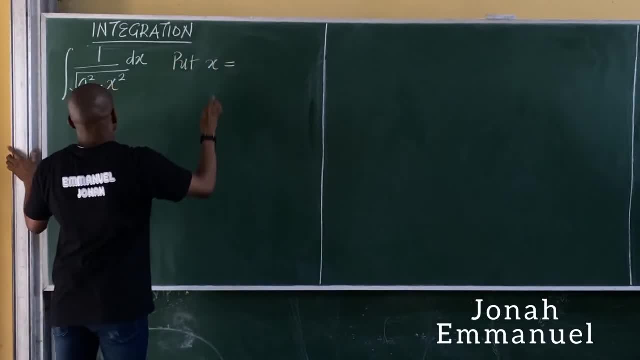 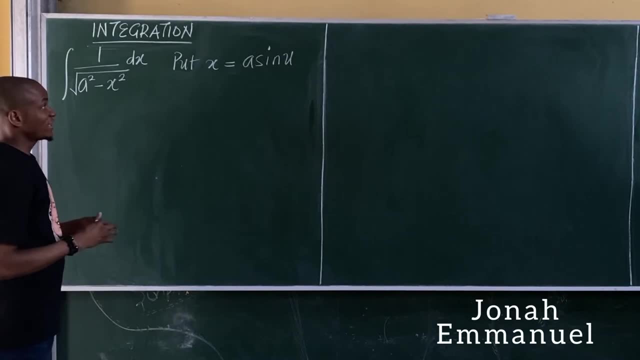 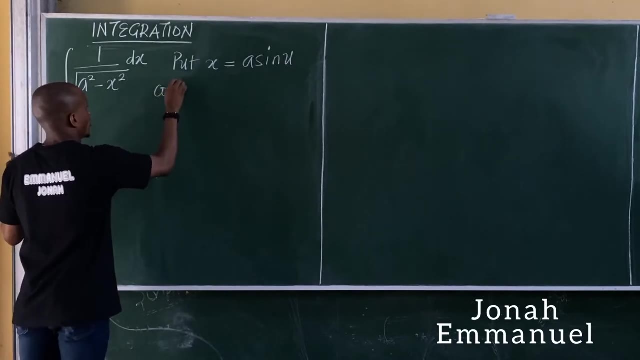 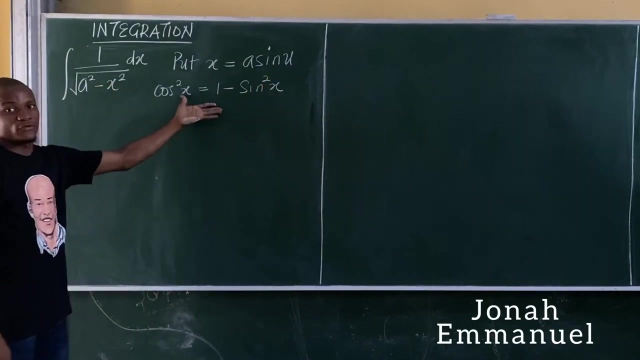 put x as u equal to a sine u. Alright, So you have this Also. for cases like this, what you should also do is this: Use the trig function that cos squared x is equal to 1 minus sine squared x. Of course, this is also from. 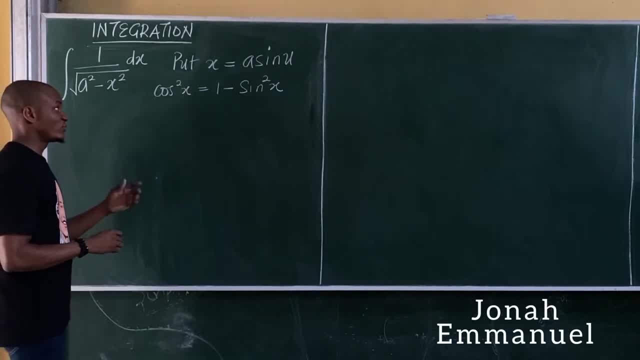 trigonometric identities. I'll also give an example here and we'll work on this. see how it works. Let's, for example, we have to evaluate the, evaluate this integral. So let's say this integral: the x all over root 16 minus x squared this case. So what do I do here? I know that 16. 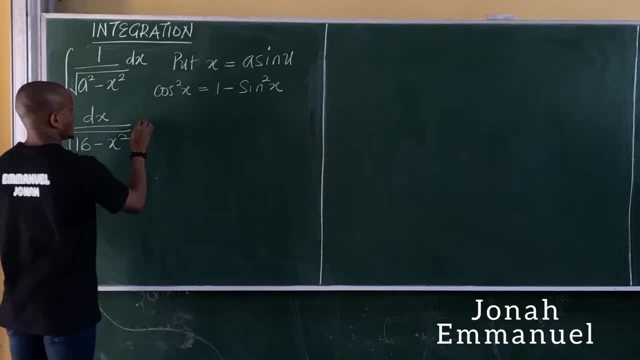 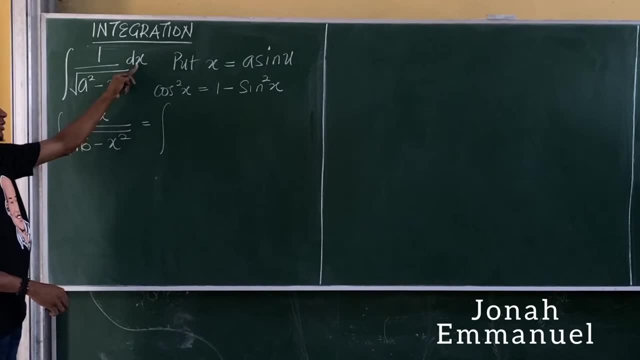 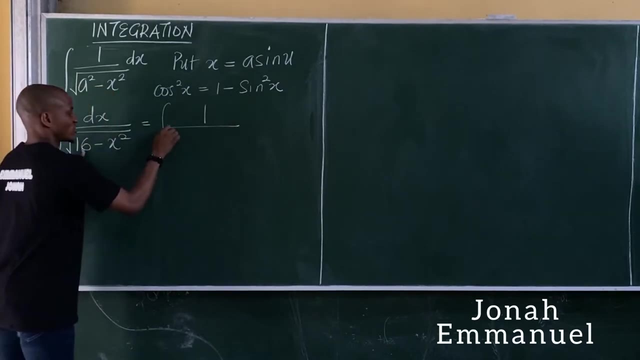 can be expressed as 4 squared, So our expression has been equal to integral. You can choose to put 1 all over. You move the x this way, just like this. okay, So I'm shifting the x this way, now I'm having 1 all over. This gives you square root of 16, as we know, is. 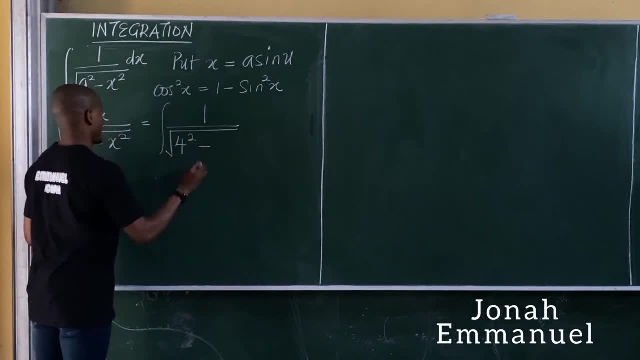 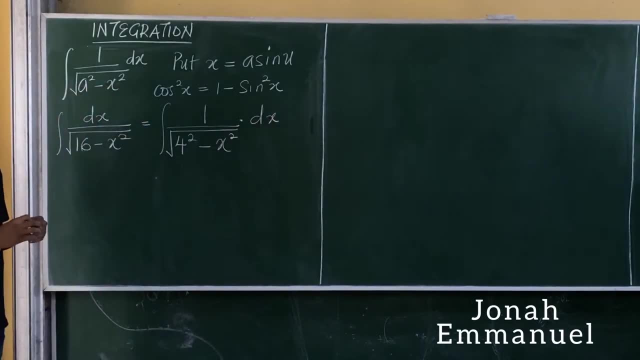 4 squared. I'm having 4 squared minus x squared dot dx. So this and this are exactly the same thing. We said for an integral of this form. we said: put x. So we'll say: let x be equal to this value here sine u. 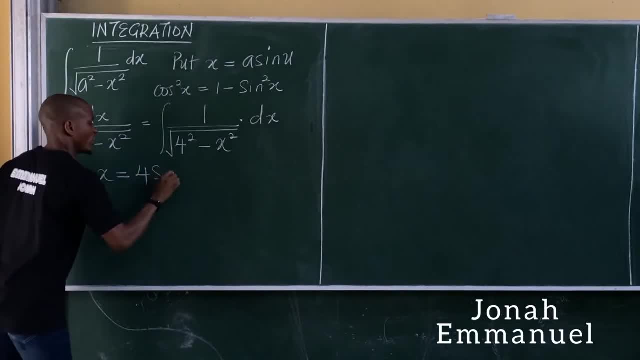 Divide here is 4.. So it becomes 4 sine u. Case 1 here. make u subject of the formula To do that there, I'll divide both sides by 4.. Divide this by 4. It gives you x all over. 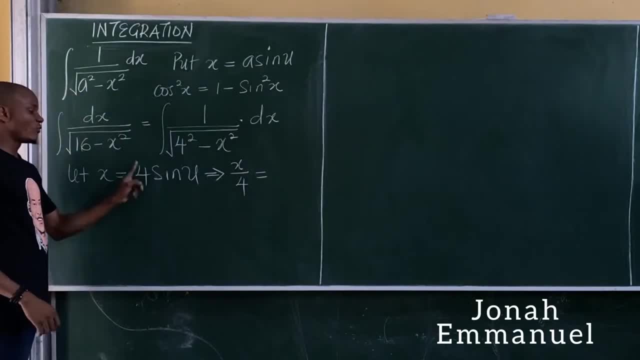 4 is equal to divide here by 4.. 4 cancels 4.. I'm left with sine u, So it's equal to sine u. I have this case here Next up to get u. I'll take the sine u. I'll take the. 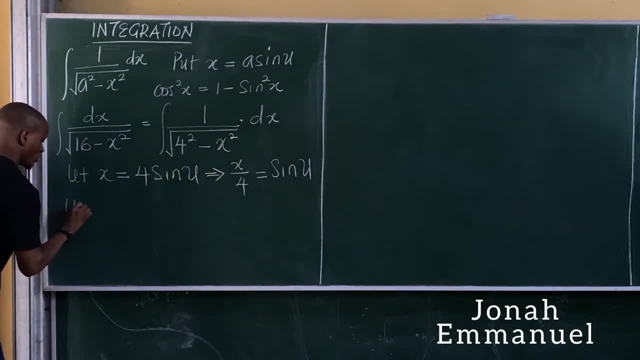 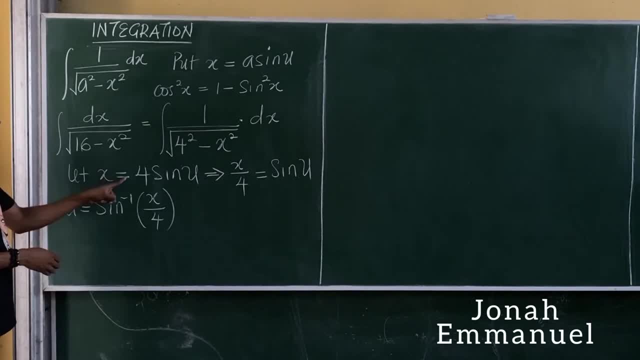 the value of u. Next up. we said x is equal to 4 sine u. If I differentiate x with respect to u, I will have that differentiate x. here we have that d x all over d. u is equal to force. it conflict 4 this wayDifferentiate 6 and. 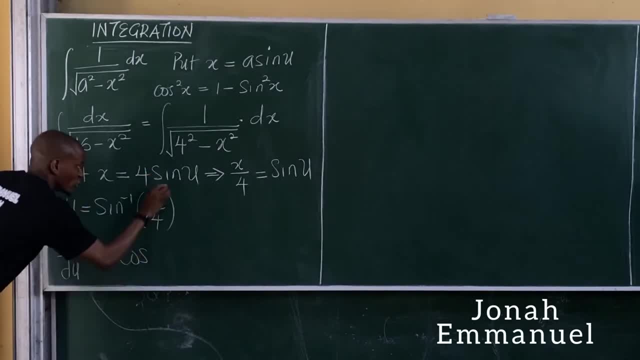 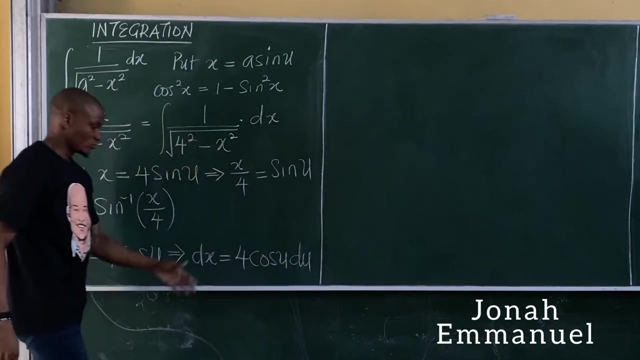 sign. you get cos, So it becomes cos of cos u. Alright, Let's get the x here. I will move the u over here, such that I will now have that the x is now equal to. if the u comes this way, I will have 4 cos u and then the u, So you have 4 cos u, the u, So I have. 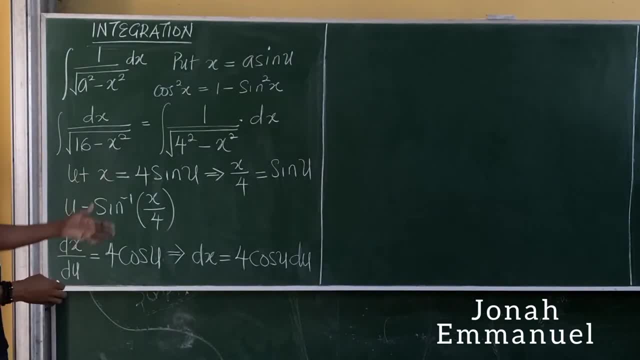 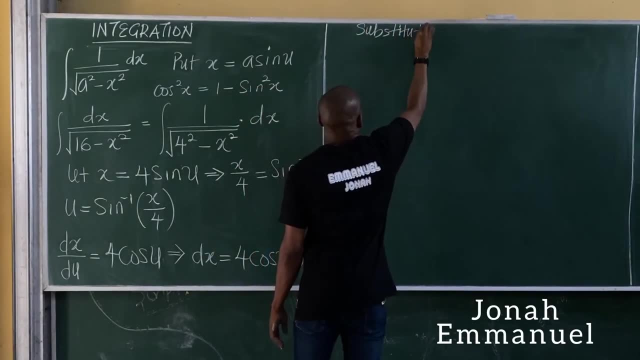 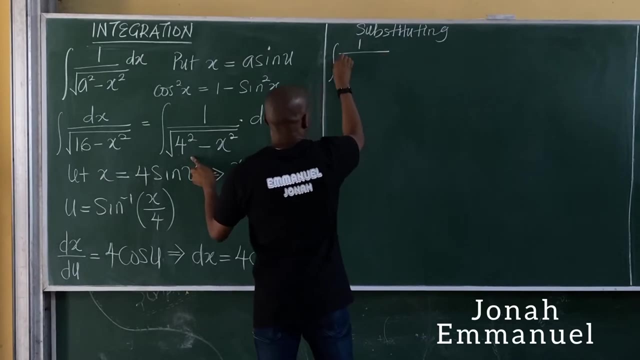 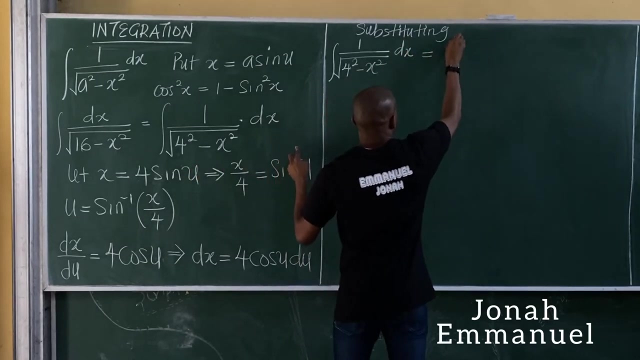 this Next up, I will substitute this value into my given function. So substituting, substituting, I have the integral of 1 all over root 4, squared minus x squared dx, as being equal to integral of 1 all over root 4.. 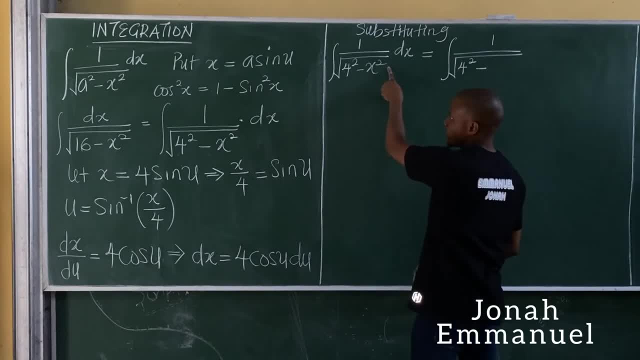 4 squared minus x squared. What is the value of x here? x is equal to 4 sin u. So in place of x here I will put 4 sin u. This becomes x all squared. So this is x squared 4 minus. 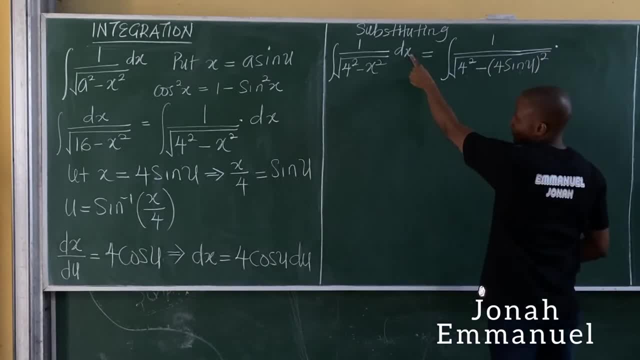 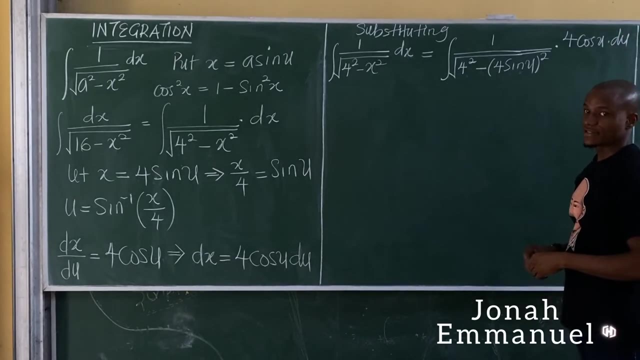 x squared, then dot the x. What is the x? The x is the value here is equal to 4 cos u to u. So in place of the x I will put 4 cos u du. Here is the value of the x. Alright, Work. 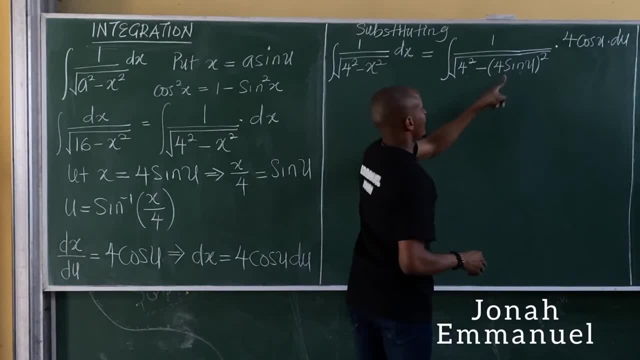 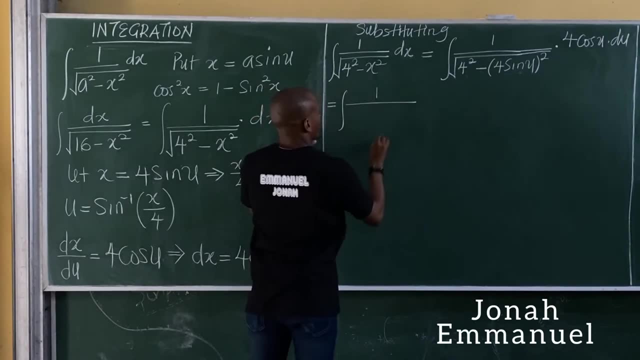 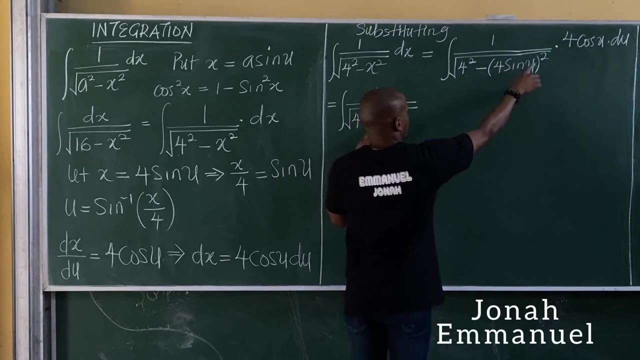 on this. now My first task is to expand this. If I expand this, I will have this as being equal to integral of 1, all over square root of 4 squared. minus from here, 4. here becomes 4 squared, So I am having 4.. 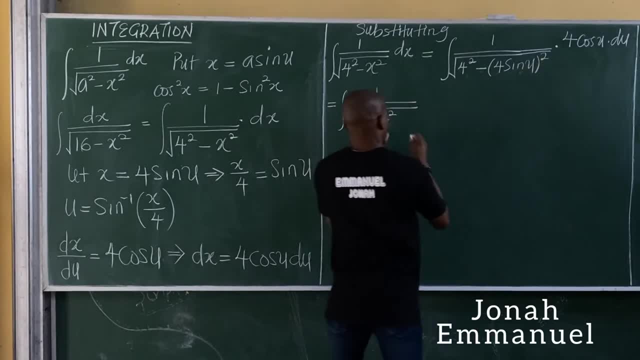 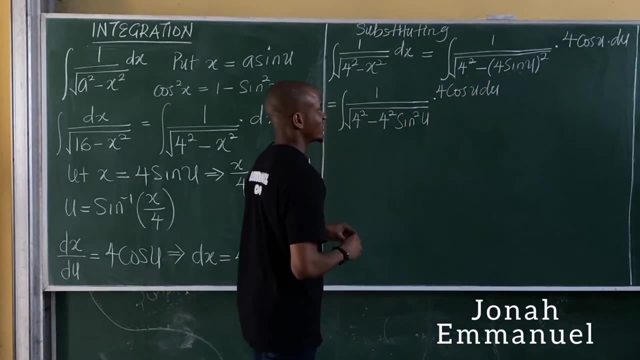 4 squared and then sin u all squared gives you sin squared u. I have this. Then dot this one here: 4 cos u du. I have this. So next up now would be to do my factorization. If I factorize this, I can see this as being: 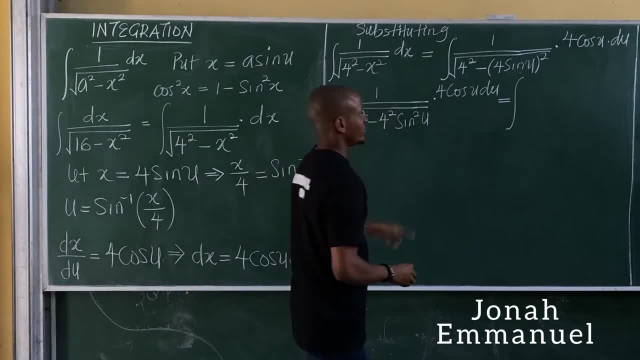 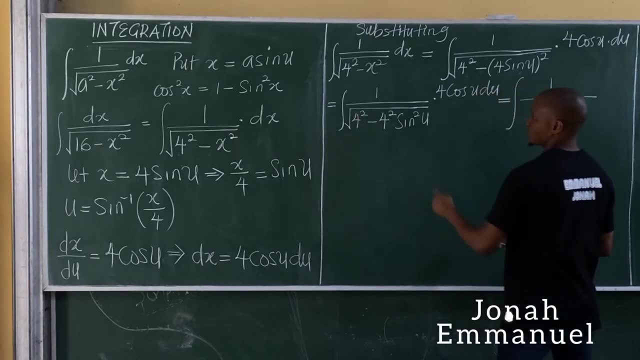 the integral of 1 all over, So 1 all over. This gives you the square root. This is 4 squared, 4 squared. So I am having square root of if I take away 4 squared, if I factorize 4 squared, I will. 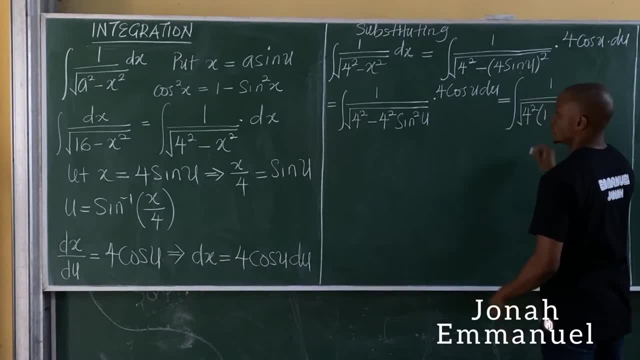 have 4 squared, there being 1.. So 4 squared over 4 squared gives me 1.. 1 minus 4 squared. sin squared u all over 4 squared. It cancels out I am left with sin squared, So this: 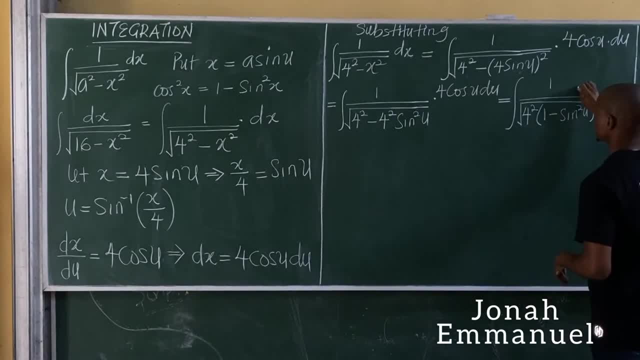 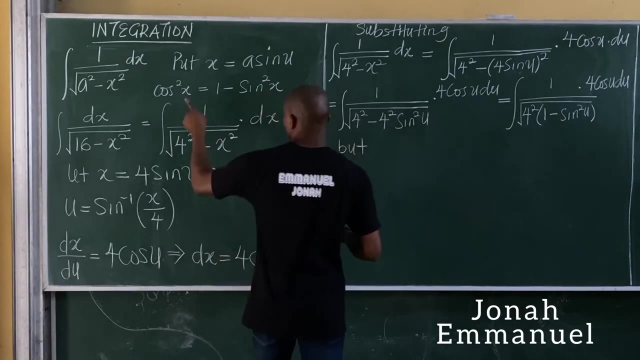 through 1, and this is pi over min squared. I have now divided here times sin squared u. So 5 squared plus 2 squared minus 1 square u. So this does here, for cos u du, 4, cos u du. So I have this. 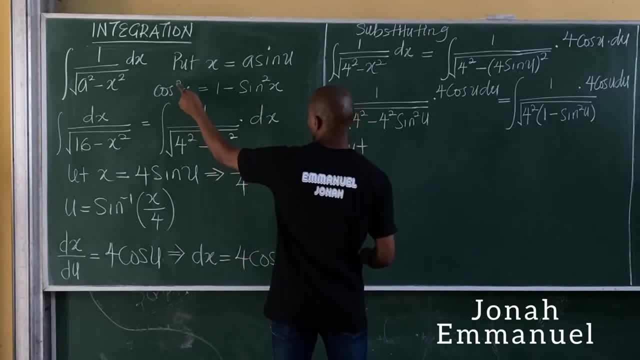 All right, So look on this now. Many of you know what this formula is. We already said that cos squared x is equal to 1 minus sin squared x. If I use u, I will have that cos squared u, but cos squared u is equal to 1 minus sin. squared u. Also, if I use sin squared u, I will have 1 minus sin squared u and sin squared u. I am re-multiplicating you and look me here. Saint is, Lacan, To寧 and Qued以上, all of. 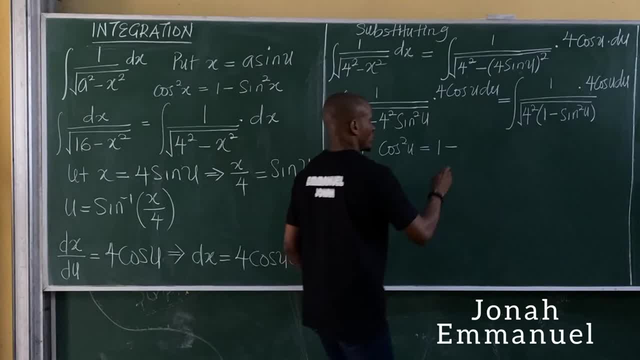 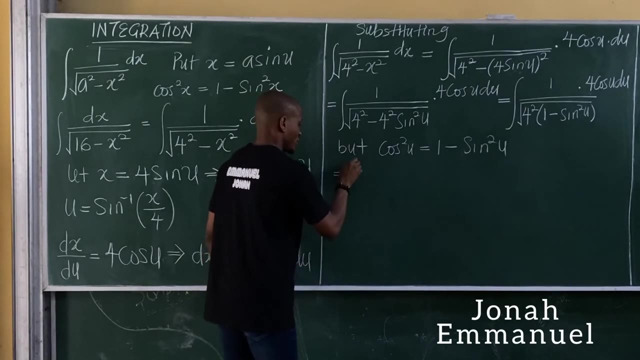 1 minus sine squared u, that's sine squared u. So I will substitute the value of 1 minus sine squared u as cos squared u And I'll be having this as being equal to the integral of 1 all over square root of 4 squared. 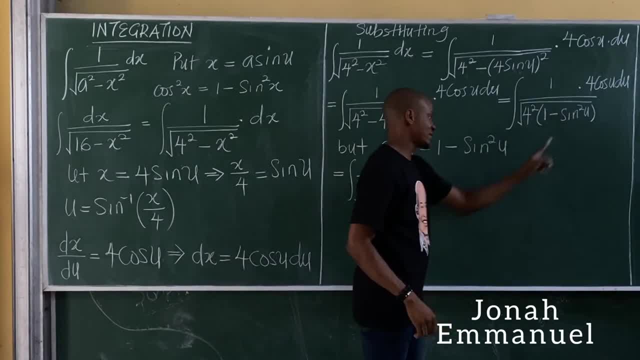 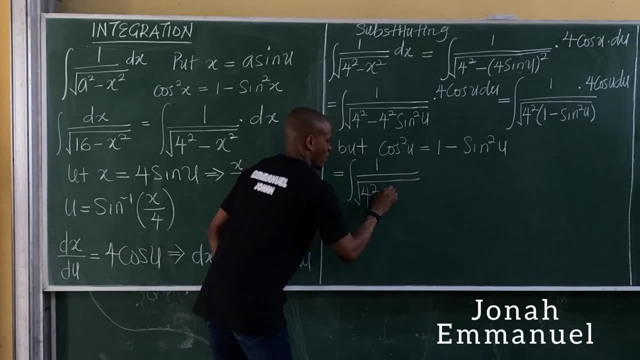 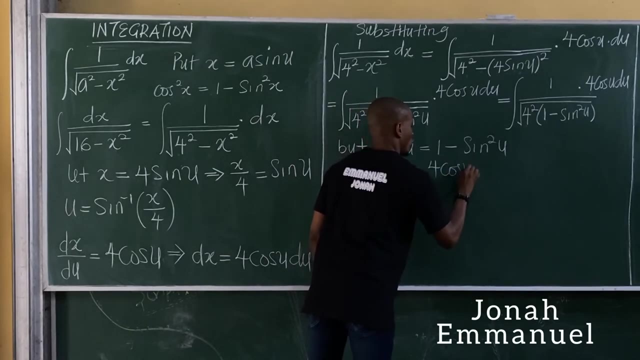 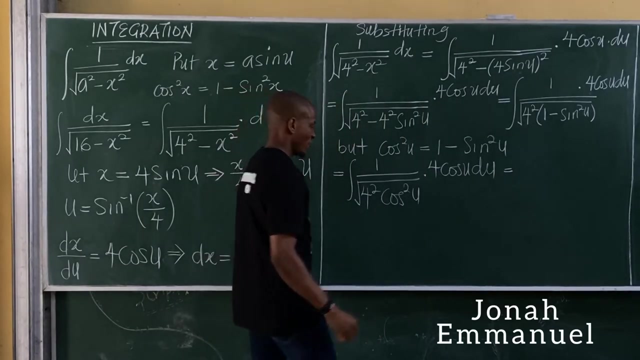 In place of 1 minus sine squared x, I'll have cos. In place of 1 minus sine squared u, I'll get cos squared u. So I'll have cos squared u here. dot 4, cos u du In this case. now, this will now be equal to: from this, I'll be having the integral of cos 1 all over. 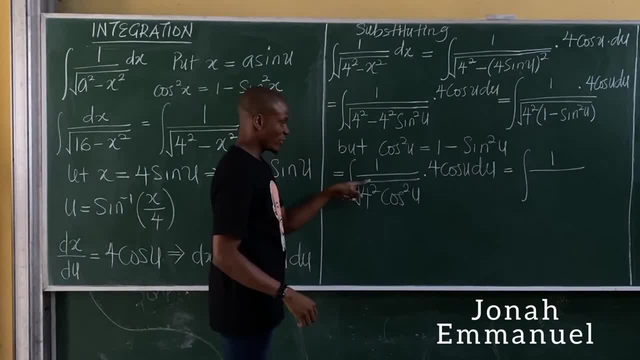 So 1 all over In this case. now the square root here will cancel this square. also, square root here will cancel this square. So it's more like saying: this is 4 cos u all squared, So hence the square root will cancel square root unless it's just 4 cos u. 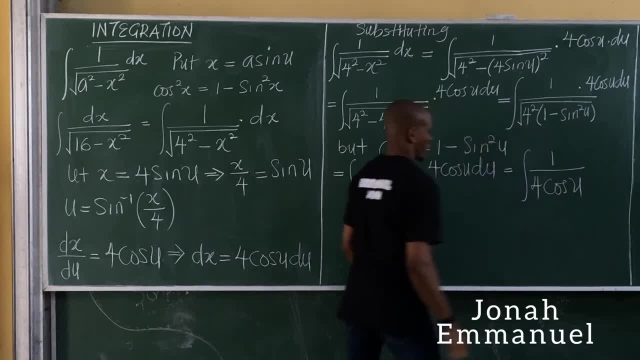 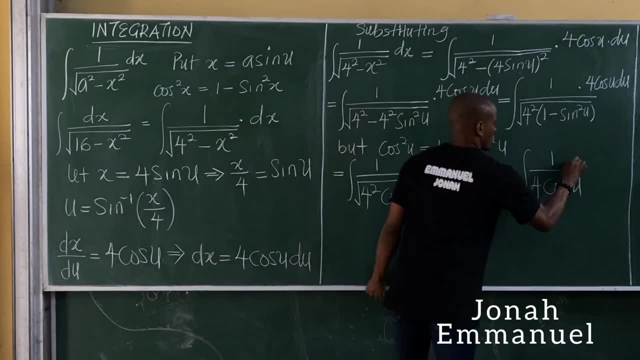 So I'm having 4 cos u here, right? So this square root will cancel both squares and it's off. So I'm left with 4 cos u dot. this is now 4 cos u du. 4 cos u du. 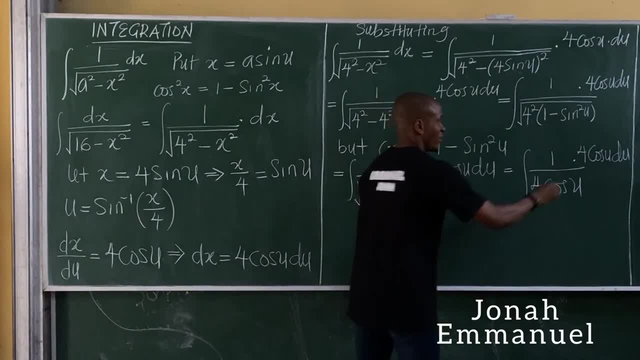 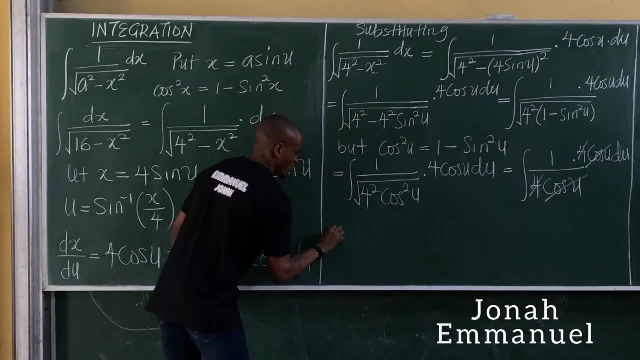 Here. 4 will cancel 4, cos u will cancel cos u. Alright, so I'm left with this being equal to the integral of 1 times u. right, This is 1 times du. that is u du. If I integrate du, I'll get u plus c. 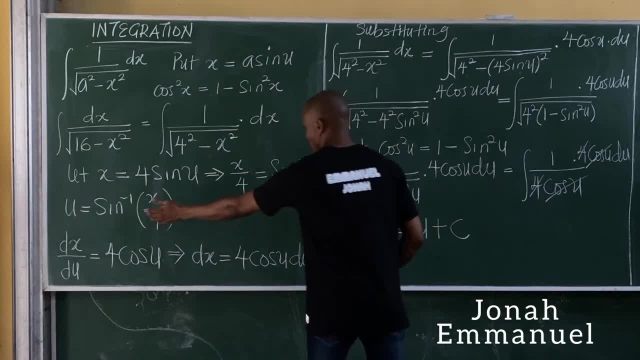 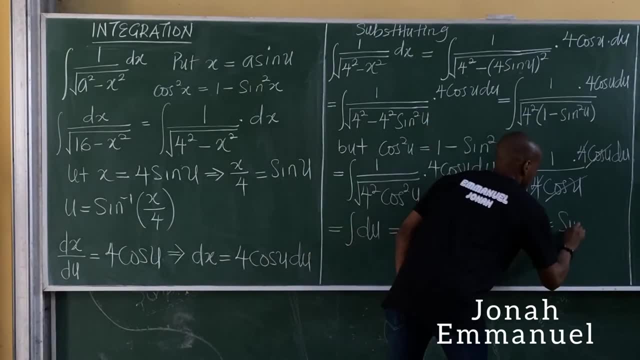 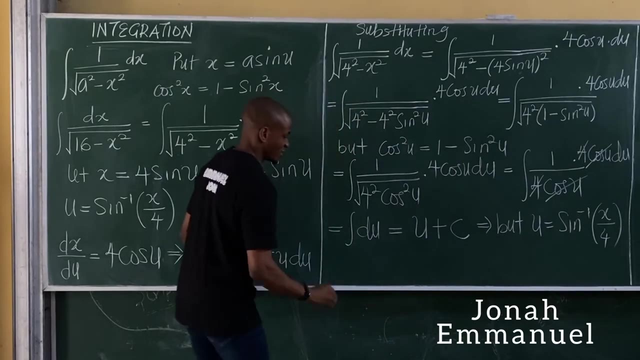 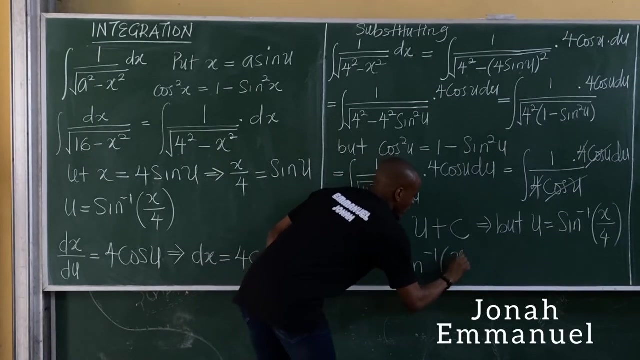 But what's u? But what's u? Okay, so we have here. but But we said u is equal to sin inverse of x all over 4.. So x all over 4.. Hence my final answer is now equal to: we said u. u is sin inverse of sin, inverse of x all over 4, that's u plus c. 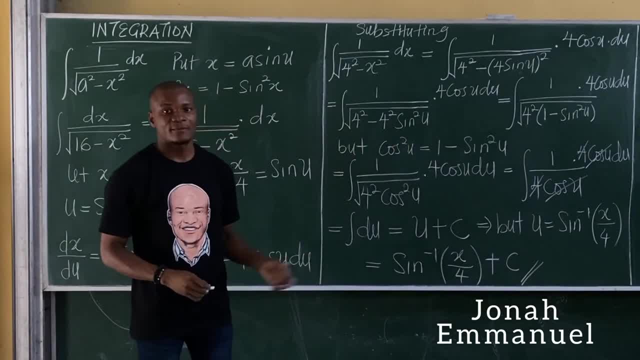 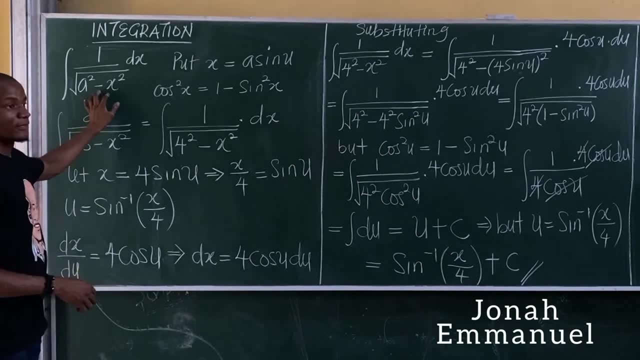 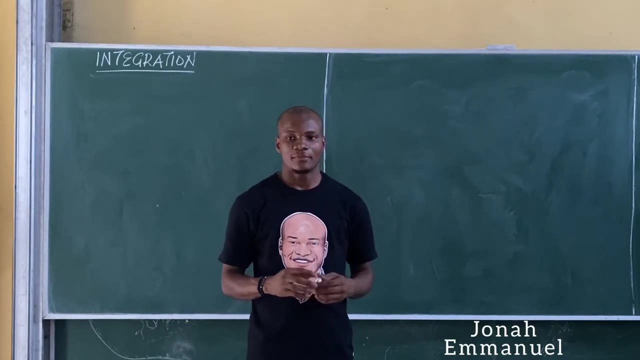 So plus c- This becomes my answer- after integration. So this is how you integrate. So this is how you integrate problems of this form. Okay, let's look at a final case of method of substitution involving trig function. The last case is this: 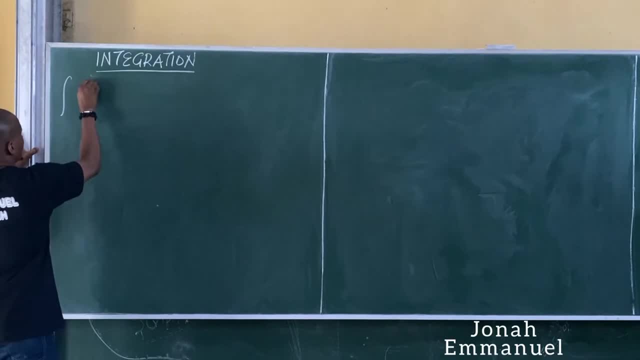 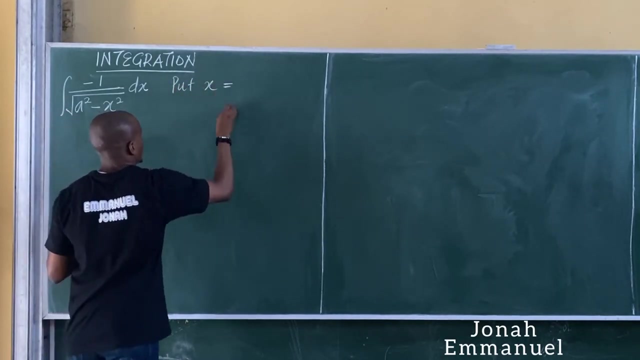 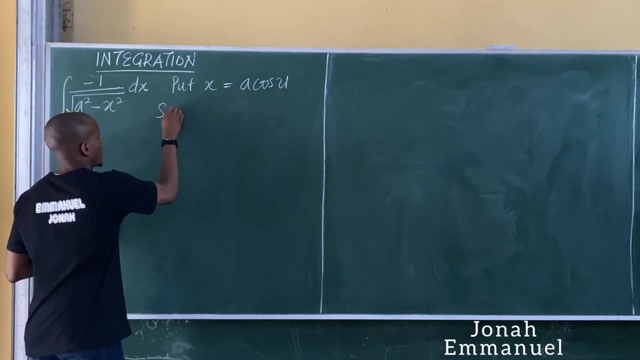 If I'm asked to evaluate an integral of the form minus 1 all over root, a squared minus x, squared, of course, with respect to x. In this case. now put Put x as equal to a cos u and also use the trig function that sin squared u is equal to 1 minus cos squared u plus x. sin squared u plus x is equal to 1 minus cos squared x, as the case may be. 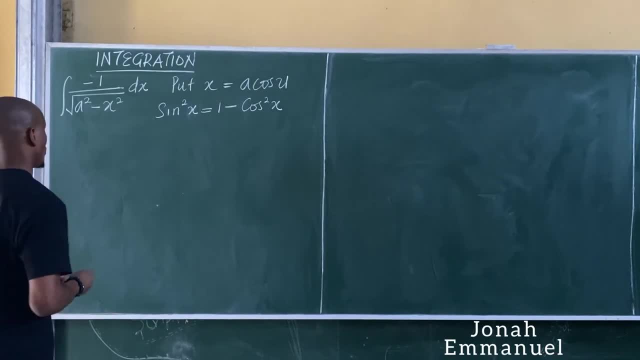 All right, so I have this. We'll take an example and work on this. Let's say I'm asking. By the way, observe: This one now is similar to the previous example. The only difference here is that there's a minus. 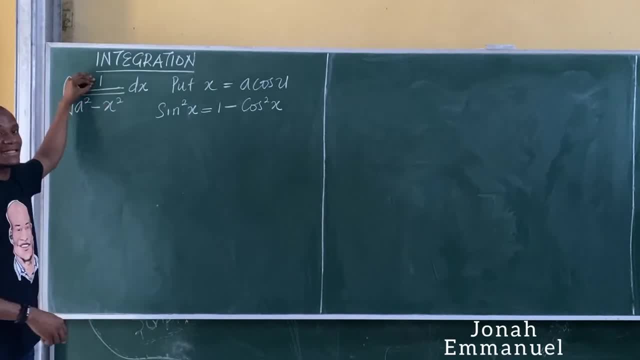 All right, that's the difference. So if there's no minus here, put x as a sin u. If there's a minus there, put x as a cos u. It's that easy, All right, Let's say we're asked to evaluate the integral. 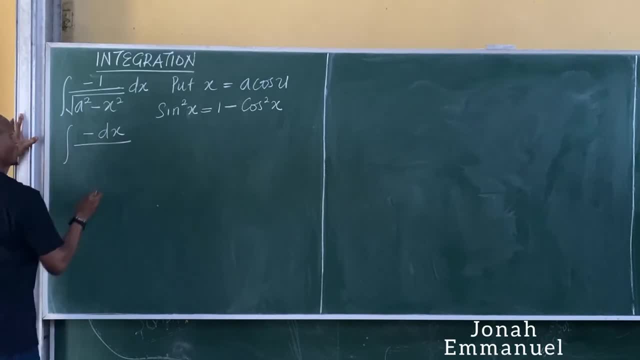 Integral of minus the x, all over root, 25 minus x squared. All right, Mark it, Integrate or evaluate this integral, The first part of this. If I look at this, I can see negative. I can see square root of 5.. 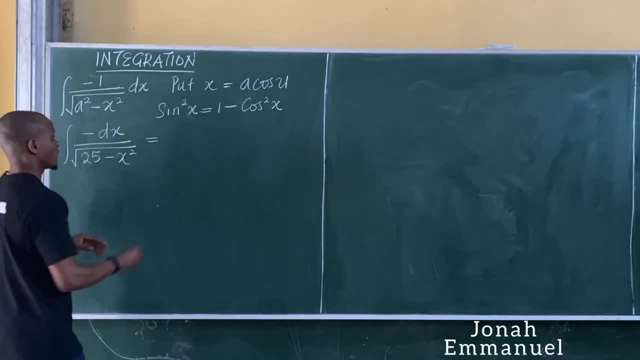 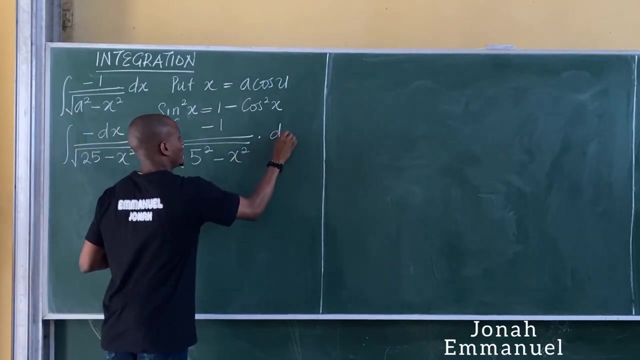 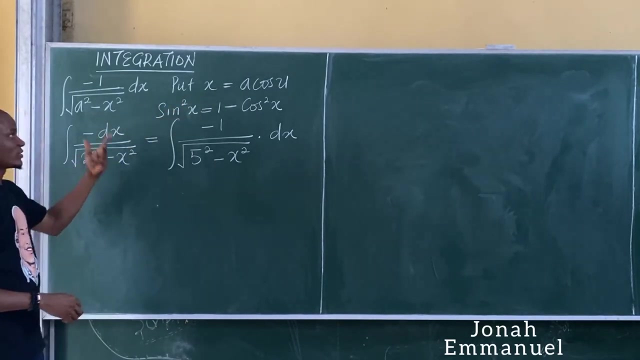 I know that 25 is 5 squared, So hence this becomes the integral of minus 1 all over root. 25 is 5 squared minus x squared dot dx. So I have dot dx, So I have dx Next up. we said: put x as a cos u. 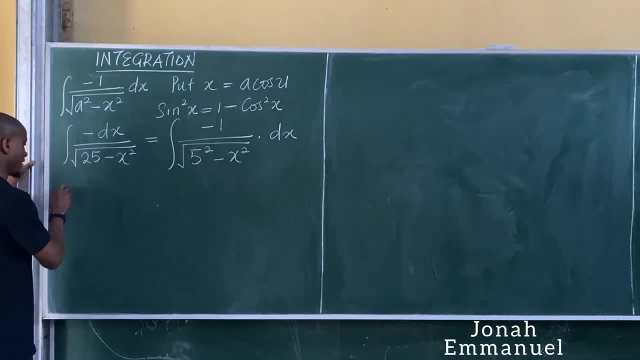 So x becomes a. In this case now it's 5.. So put x as equal to 5, cos u Let's get u again. So in this case, now for us to get u, the first task is to divide both sides by 5.. 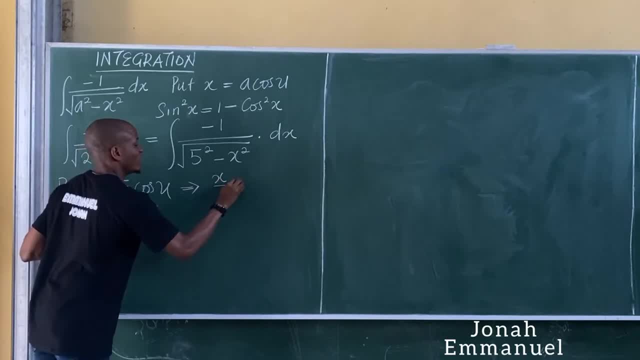 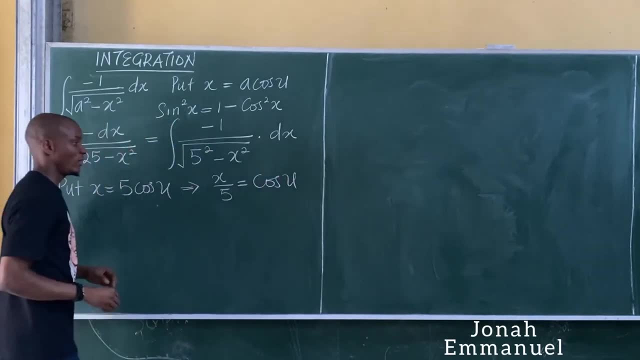 Divide x by 5. We get x all over. 5 is equal to Divide this by 5.. I'll get cos u, So I'll have cos u. All right, Next up, make u subject of the formula here. 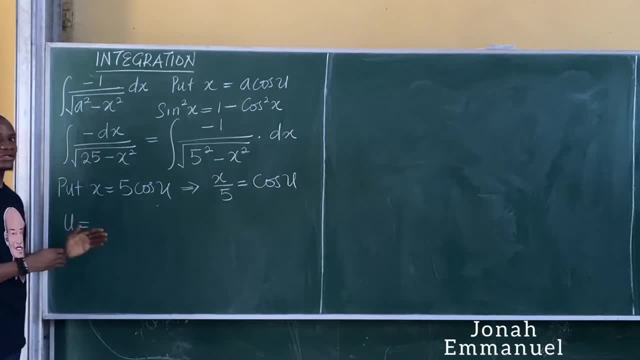 u will now be equal to. I will have to take cos inverse of both sides. It becomes cos inverse of x all over 5.. I have this All right. So this is now the value of u In this case. now if I shift x here, 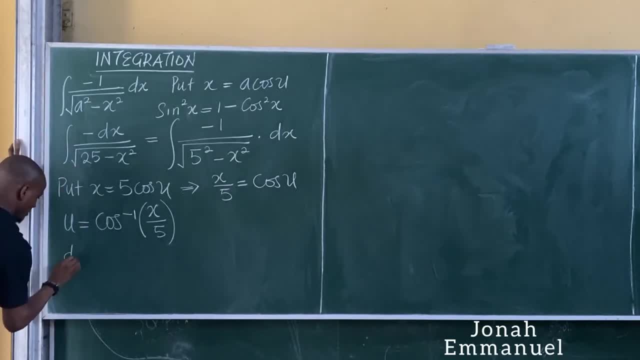 If I shift x here, I'll get. If I shift x here, I'll get the x all over. the u is equal to: This is 5.. So I'm having 5.. If I shift cos u, you get minus sin u. 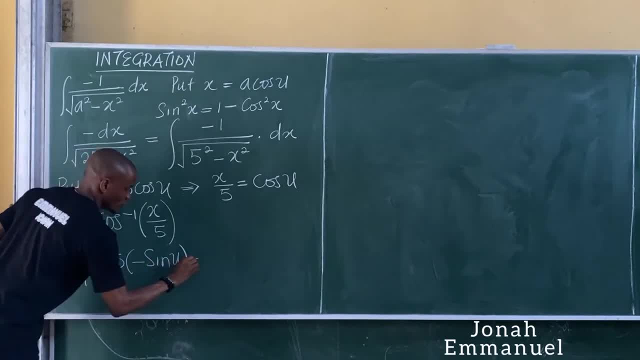 Such that I'll now have that the x by the u, The x all over the u, is now equal to minus 5 sin u. So I'm having minus 5 sin u. Let's get x here. Move the u over here. 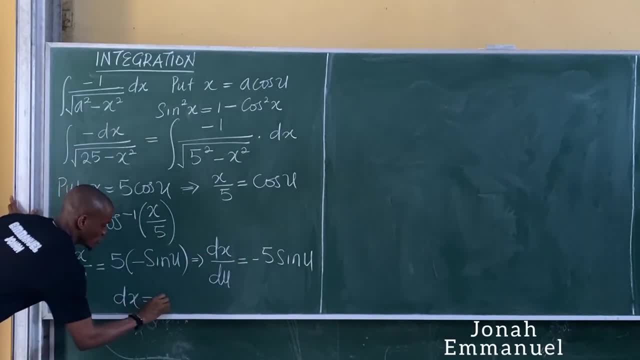 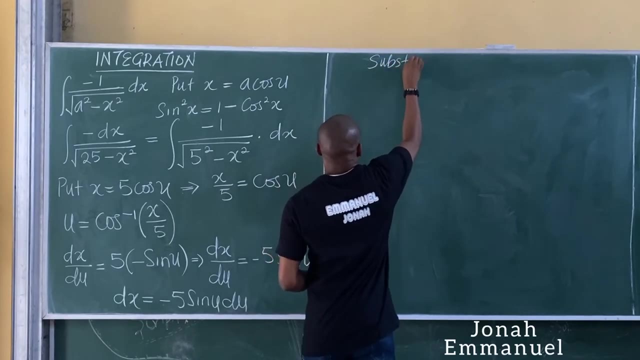 So it means that the x is now equal to minus 5 sin u du. All right, The x is now equal to minus 5 sin u du. After making this next up, I'll do my substitution, So substituting. 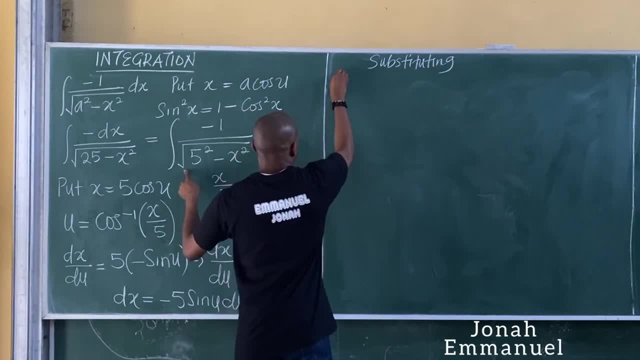 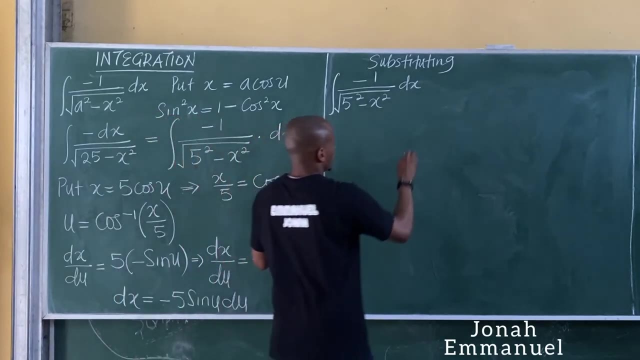 If I substitute now, the equation was this: The integral of minus 1 all over Roots, 5 squared minus x squared dx. So the substitution is here: This will now be equal to the integral of minus 1 all over roots. 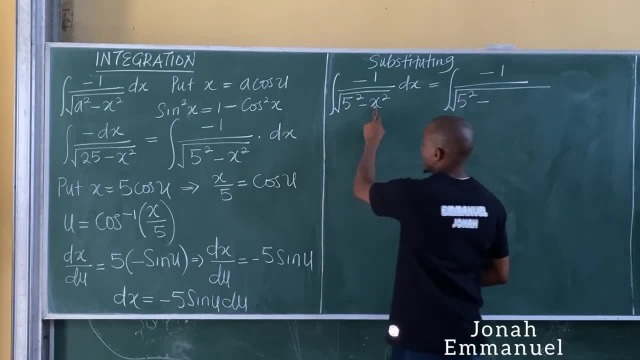 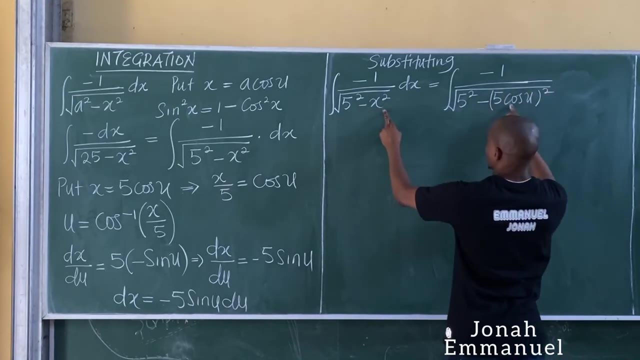 This is 5 squared minus x squared. What's x? We said x here is equal to 5 cos u. So we got 5 cos u. This is x, all squared, All right. So 5 squared minus x squared, dot dx. 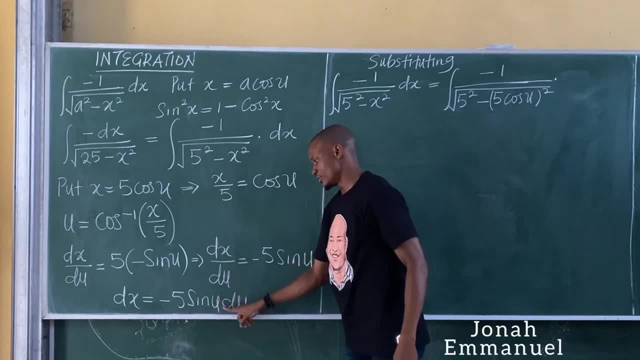 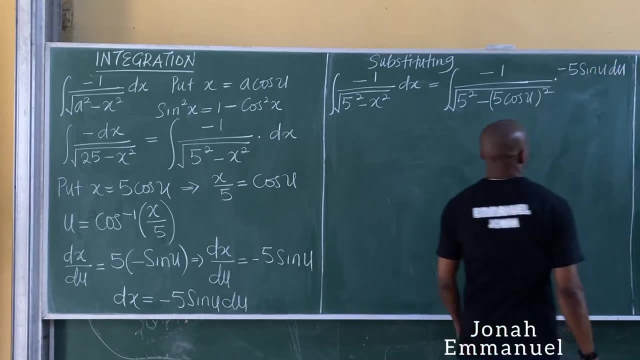 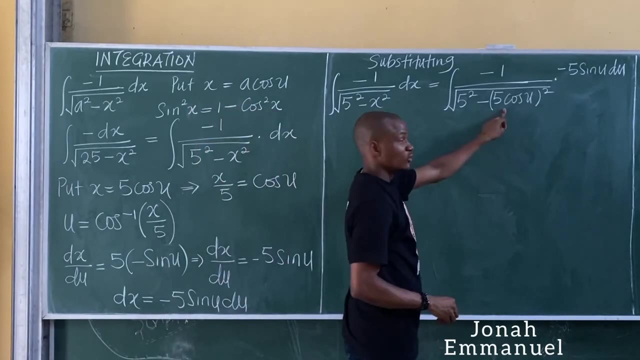 The x here is minus 5 sin u du. It becomes minus 5 sin u du. All right, So I have this Now. what about this? What do you get? The first task is the expandings, So this will now be equal to: 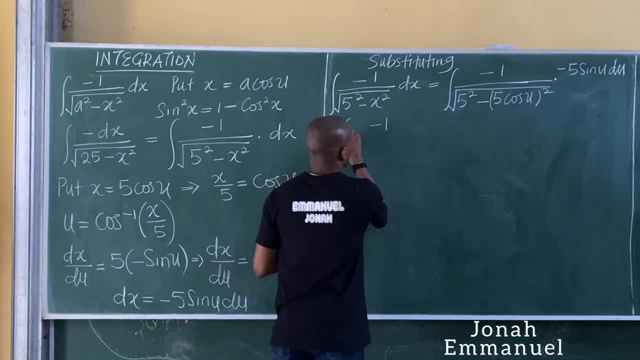 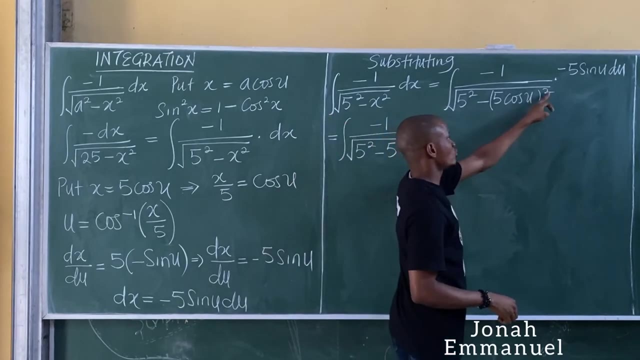 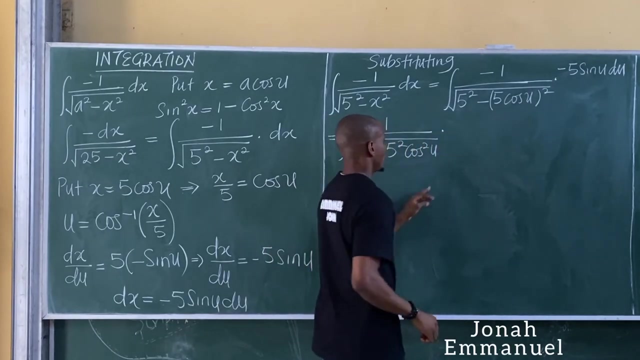 The integral of Minus 1 all over roots. This gives you 5 squared, So 5 squared minus. If I expand this 5 to this gives you 5 squared. I'm having 5 squared into cos u squared gives you cos squared u into cos squared u. dot multiplying minus 5.. 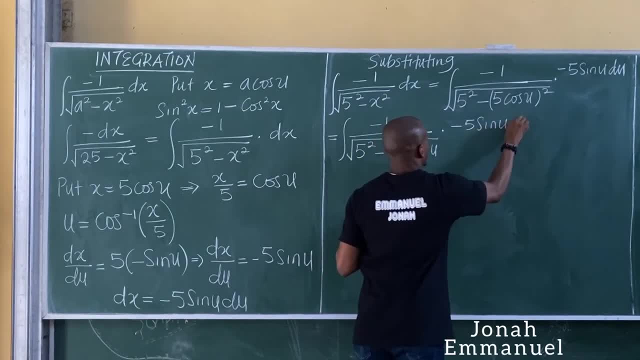 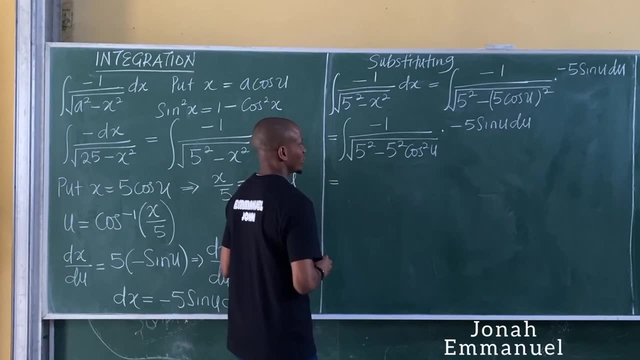 So minus 5 sin u du. I have this In this case. now, if I multiply 2, this will now be equal to the integral of minus 1 times. This gives you minus, Minus. minus is plus, So I'm having plus 5 sin u. 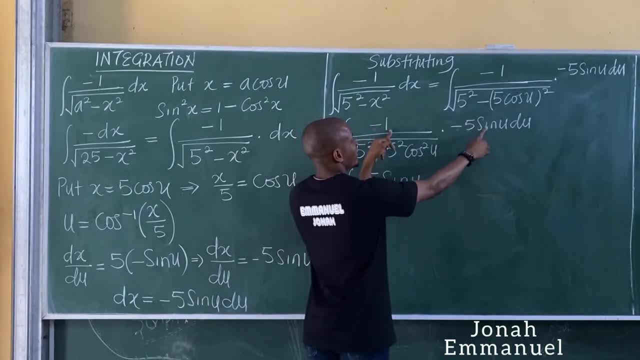 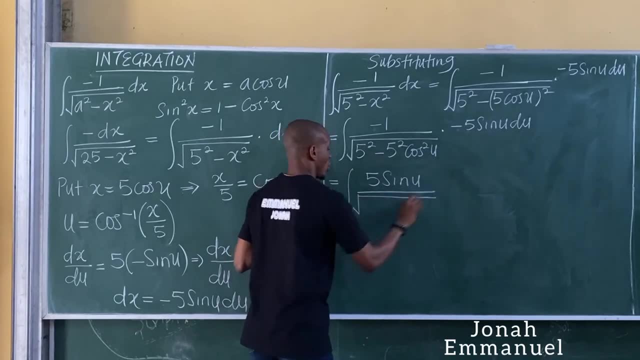 Minus times 1 gives you plus 1 times 5 gives you 5. sin u, So sin u all over. If I factorize it before, then Square root of Square root of I'm having 5 squared, I'm having 5 squared. 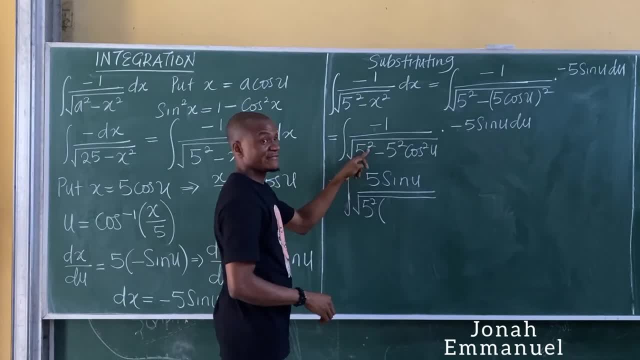 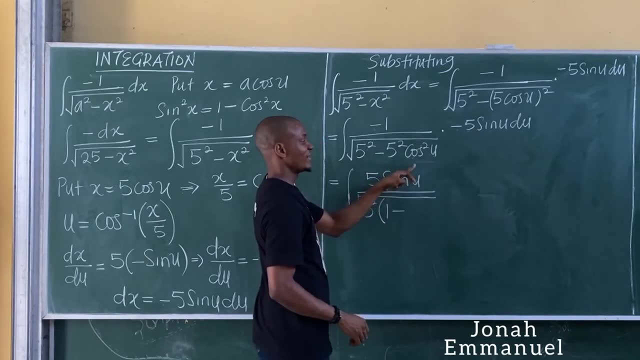 So factorize 5 squared here. 5 squared divided by 5 squared gives you 1 minus 5 squared cos squared u divided by 5 squared, 5 squared plus 5 squared, I'm left with cos squared u minus cos squared u. 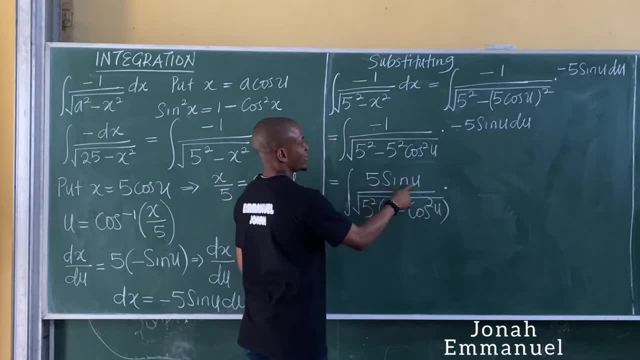 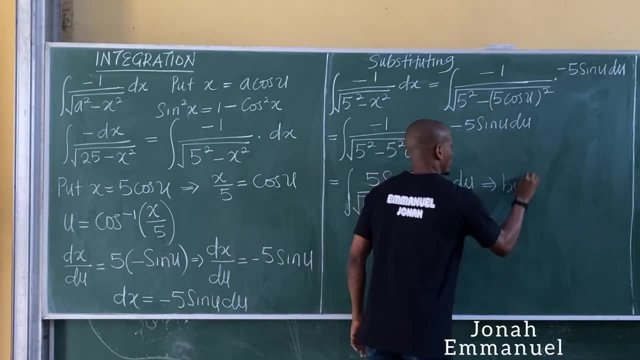 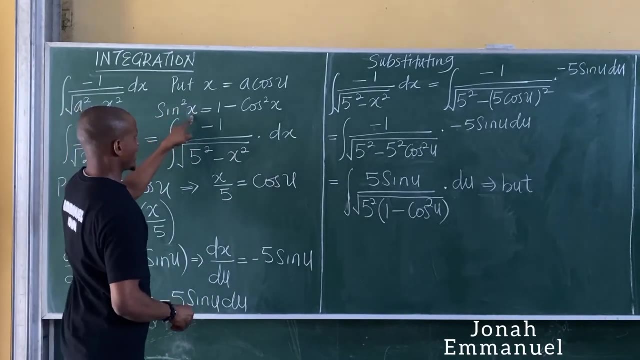 This times This was 5 sin u, 5 sin u. I'm left with du, Alright, But, But. But We said that. What is it? We said that sin squared x is equal to 1 minus cos squared x. 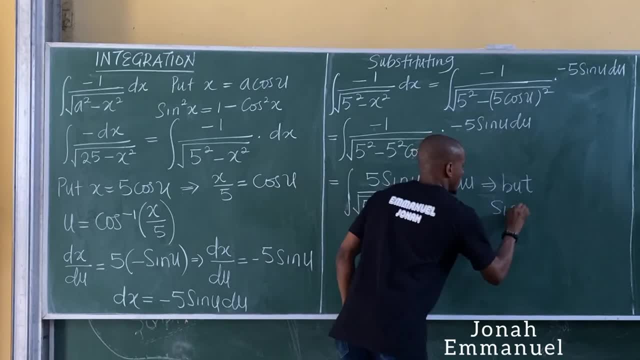 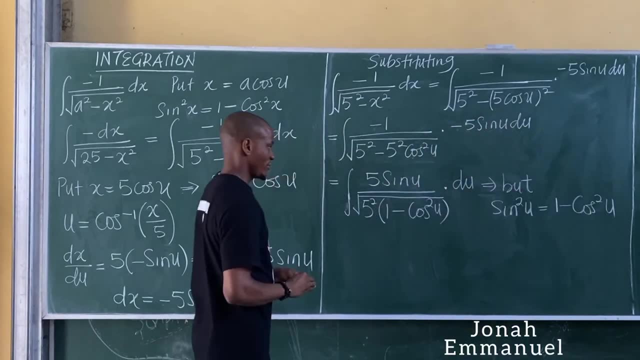 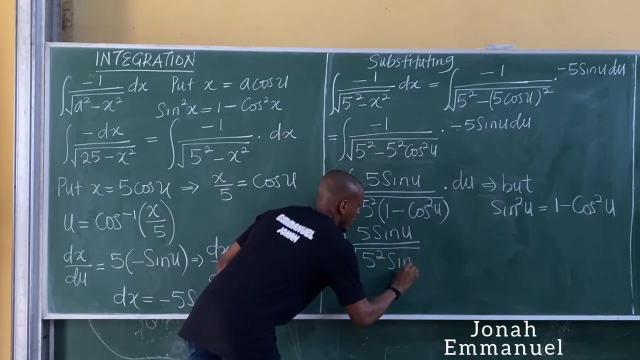 That means sin squared u, but sin squared u is equal to 1 minus cos squared u. Okay, So in place of 1 minus cos squared u, I'll put sin squared u. This will now be equal to: This will now be equal to the integral of 5 sin u all over square root of 5 squared into 1 minus cos squared u is sin squared u.